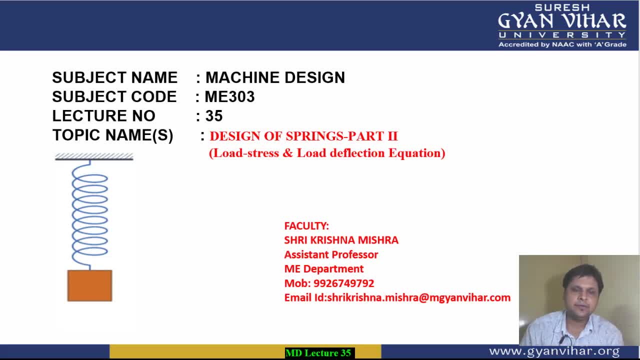 Hello and welcome students. We are into the 35th video lecture of the video lecture series made on the subject of machine design, whose subject code is ME303, and the topic which I am going to discuss with you today is the design of spring, part 3.. 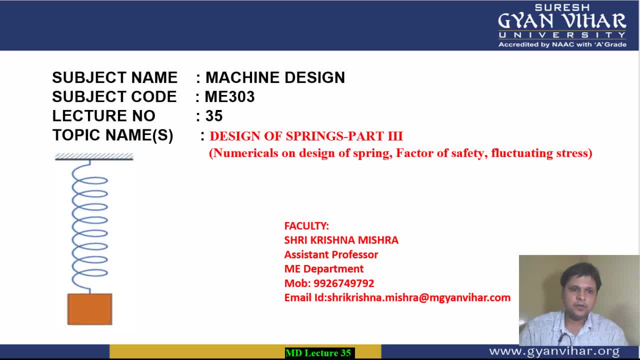 So majorly in this third part of the design of spring we are going to discuss about the different numericals on the design of spring Theory, the two equations which are important for the design of spring, that is, the load stress equation and the load deflection equation. 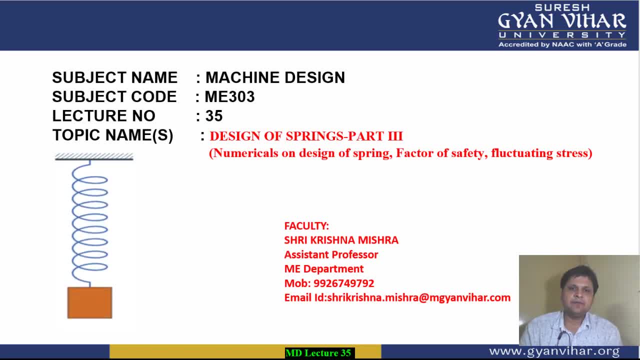 we have already derived it in the previous video lecture Alright. so based on those two equations, we are going to design the springs. means we are going to solve numericals in which we are asked to design the spring. Also, the factor of safety is very important consideration that has to be taken in the case of a spring. 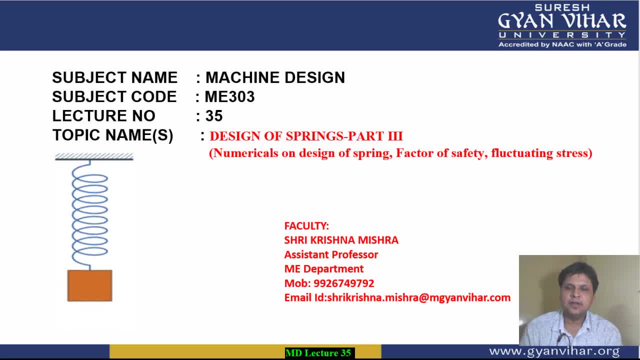 also. So we will see what are those factor of safety values and then that one more thing that is important as far as the design of spring is concerned is the fluctuating stress. that is the fluctuating stress. So we are going to discuss about the fluctuating stress. 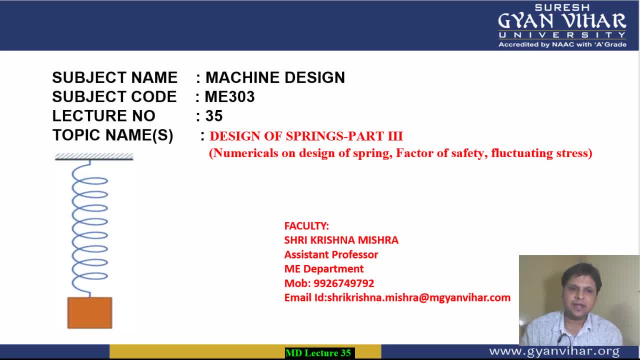 that are developed in the spring, because many a times the load that is acting on the spring is the fluctuating load. So how the spring has to be designed considering the fluctuating load. that also we will see. So before this, if you have not seen my previous. 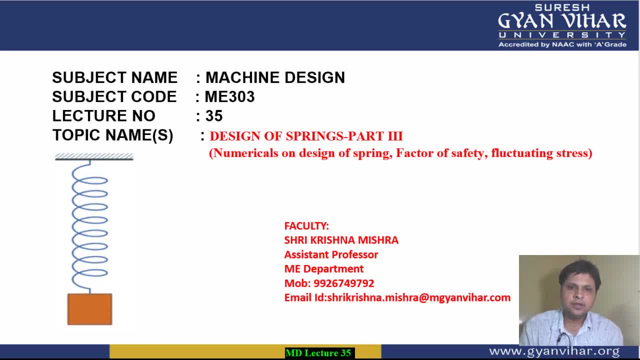 video lectures on this particular topic of design of spring. go and watch those video lectures. It will be beneficial for you. I am Shri Krishna Mishra, Assistant Professor in the Department of Mechanical Engineering, Suresh Gyan Vihar University, Jaipur. So. 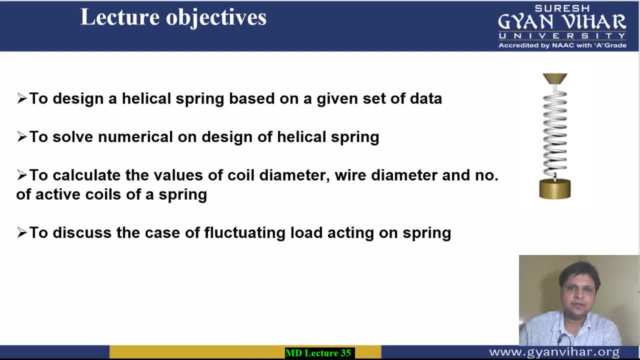 before moving into the discussion, first of all let us see what are the objectives of today's lecture. So the objectives of today's lecture are, first, to design a helical spring based on a given set of data. So basically, in today's lecture we are going to design a helical spring. 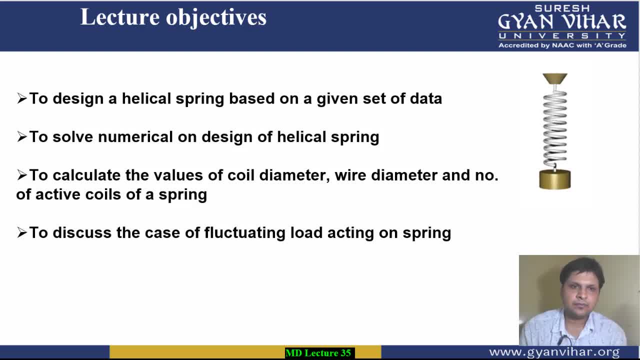 based on input values or some data has been given to us, Alright, like the load which have to be applied on the spring. So if some data has to be has been given to us and we are asked to design the spring, how we will design the helical spring we are going to. 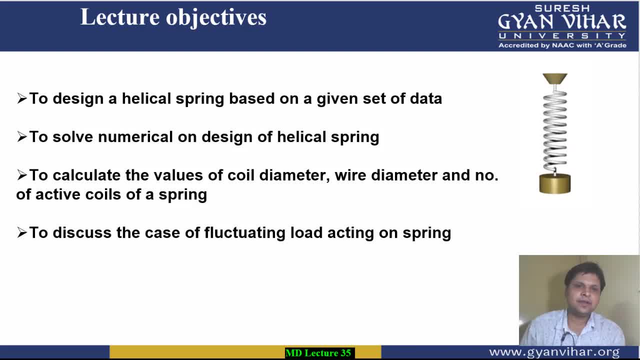 see. The second objective is to solve the numericals which are based on the design of helical springs. then the numericals which are based on the design of helical spring. we are going to solve those numericals. Then the third objective is to solve the numericals. 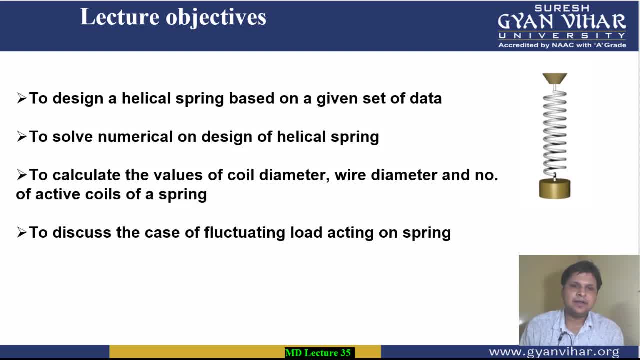 lecture objective is to calculate the values of coil diameter, wire diameter and number of active coils of a spring. Our third objective, student, is we are going to calculate the parameters which are very important in design of a spring, that is, the coil diameter, wire diameter. 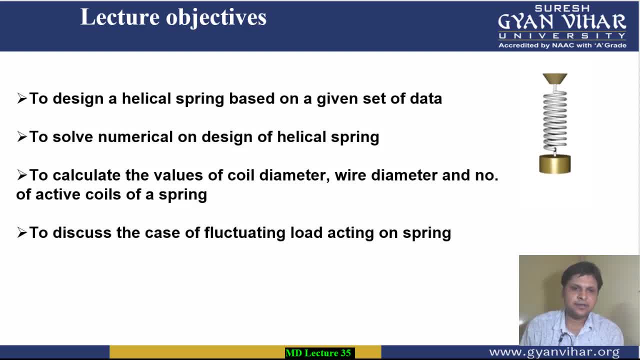 and the number of active coils of a spring. Then, after, our last objective is we are going to discuss the case of fluctuating load that will be acting on the spring. So this is the important case of a design of a spring, because many a times a spring is acted upon by a fluctuating load. So 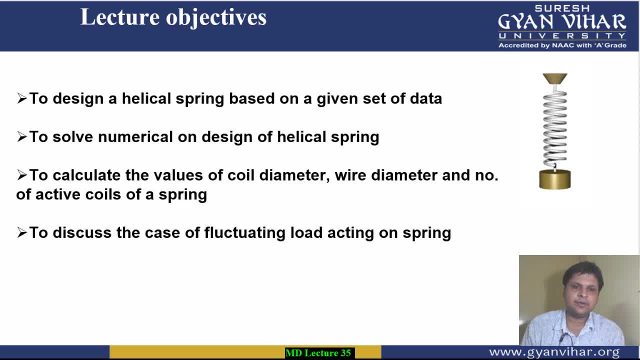 we are going to understand what happens when the fluctuating load acts on the spring and the second thing, how we are going to design the spring on the basis of fluctuating load acting on it. So these are the lecture objectives of today's lecture students. 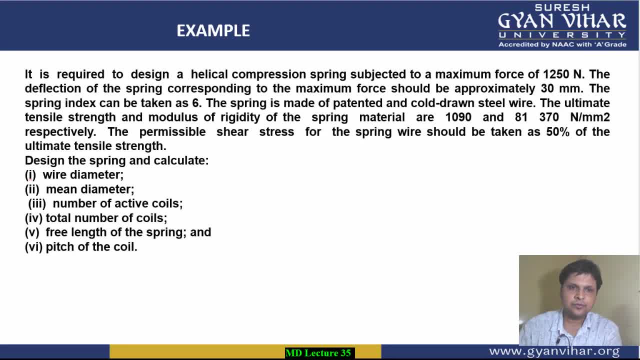 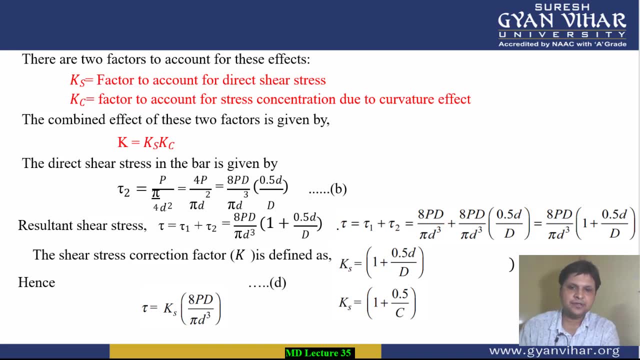 Now let us start our lecture. So this is the example which I am going to first of all consider with you in today's lecture. Now before it, in the previous lecture, we have derived the load stress equation, which is very crucial in the design of a spring. So this is the equation which 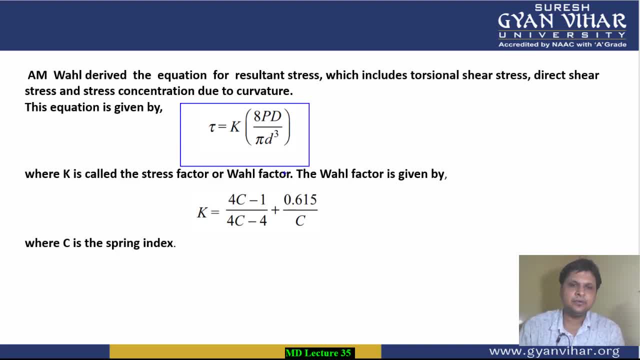 we are going to use in our numericals. tau is equal to k into 8 pd upon pi dq. Alright, this will give you the value of stress acting on the spring. and here there is a constant, there is a factor which is known as k. k is your stress factor or wall factor, and wall factor value is given by this particular. 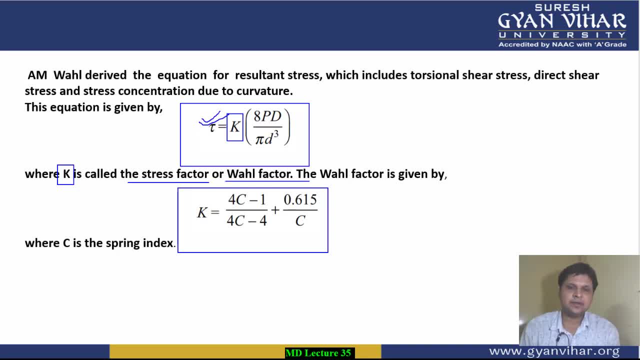 formula k is equal to 4c minus 1 upon 4c minus 4 plus 0.615 upon c. Here capital c stands for spring index. Alright, so we are going to use this particular load stress equation for calculating the coil diameter and wire diameter. 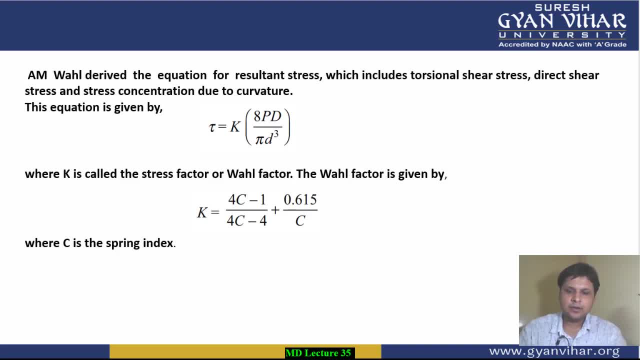 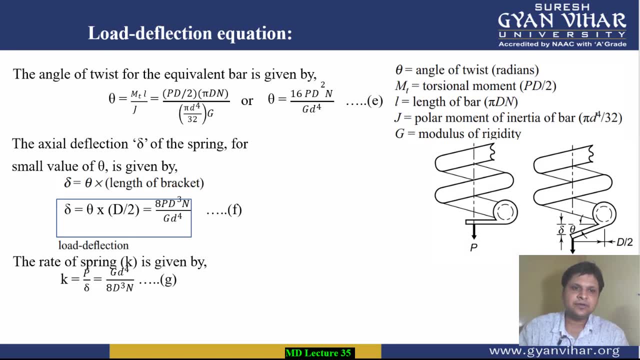 Then after students. after this: I have already told you in previous lecture, we have derived the load deflection equation also. So, based on this load deflection equation, which is given by this particular equation, that del is equal to 8 pdq of n upon gd4, we are going to calculate this n. 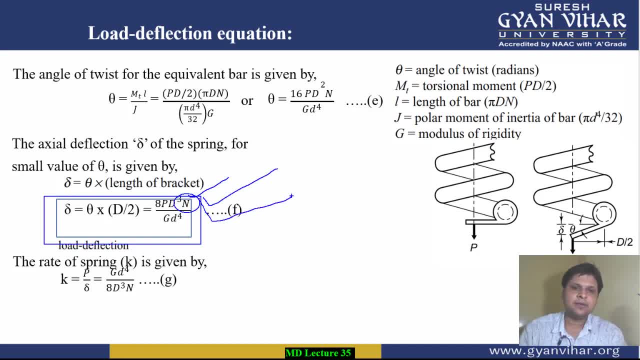 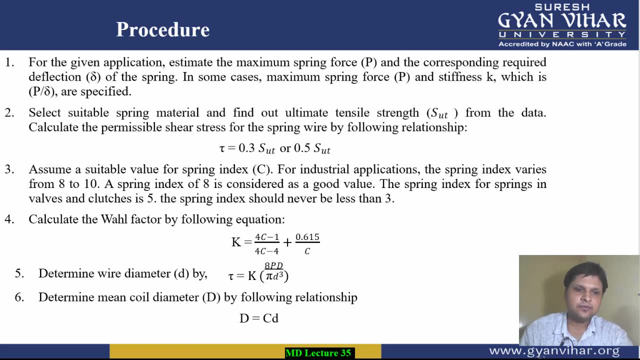 We are going to calculate this. n, n is what n is the number of active coils. So, through this load deflection equation, we are going to calculate the number of active coils. So we are going to calculate the number of active coils. Alright, then, after also the procedure of design of 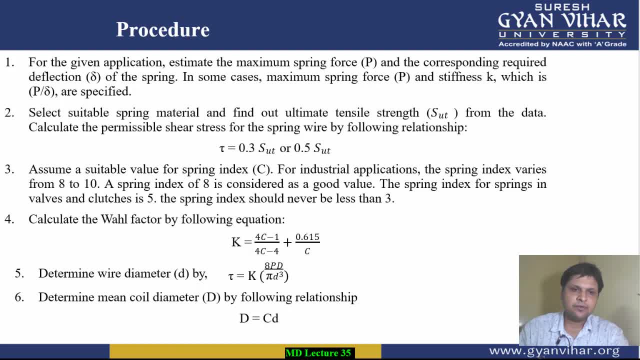 helical spring was also taught to you in the previous lecture. This was whole of the step which are to be followed. We are going to calculate the value of spring index, wall factor, wire diameter, Alright, mean coil diameter. Then after, we are going to calculate the number of active coils. So 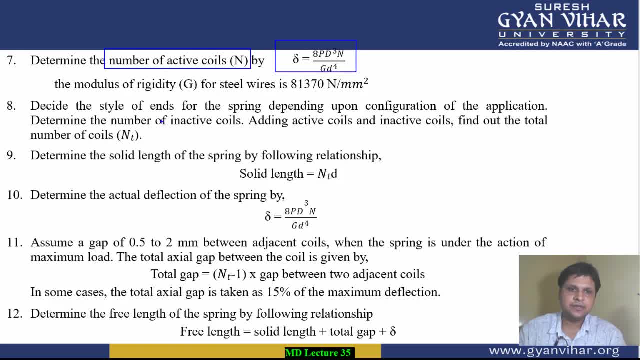 calculate the number of active coils by the load deflection equation, then how much is the number of total coils? total number of coils we will calculate on the basis of style of end, then solid length value we have. we can calculate then after then on the basis. 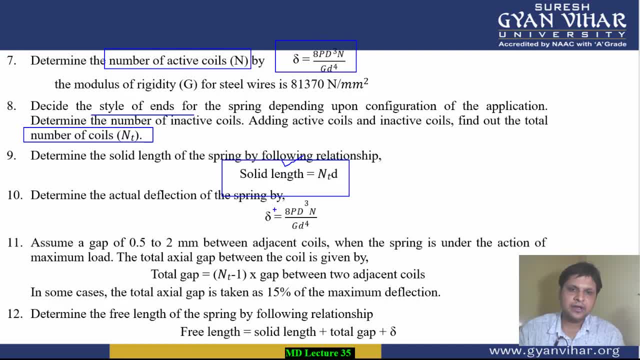 of this value of solid length and the number of active coils. again, we can use this load stress equation, load deflection equation and calculate the number of coils, Then total gap, if you want to calculate between the coils of the spring, if you want. 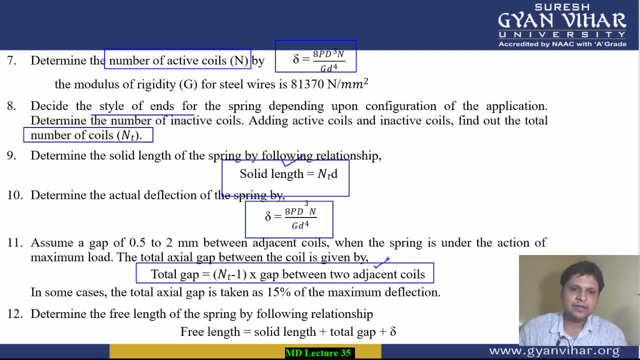 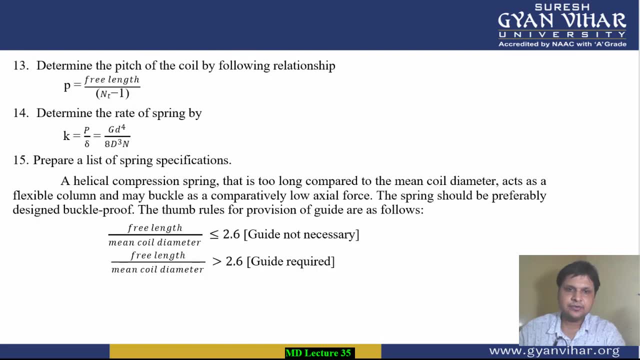 to calculate the total gap, then, by this formula, we will calculate finally, at last, the free length of the spring that we can be calculated by this particular formula, where free length is equal to solid length plus total gap, plus del. alright, so this is the equation, student. 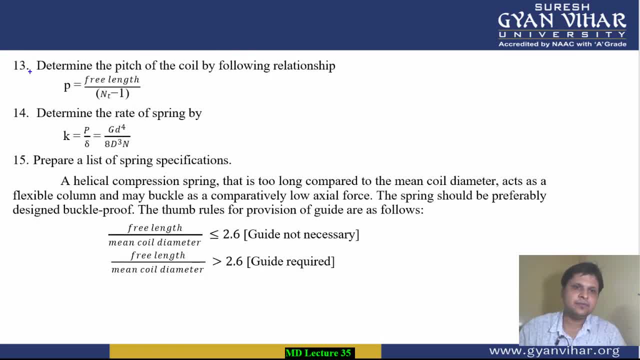 then after. apart from that, if more information is needed, then, which can also be calculated by this formula: P is equal to 0.. Which is equal to free length upon nt minus 1, and similarly, the rate of the spring that can be calculated, k is equal to p by del, and it is equal to gd to the power 4 upon 8d cube. 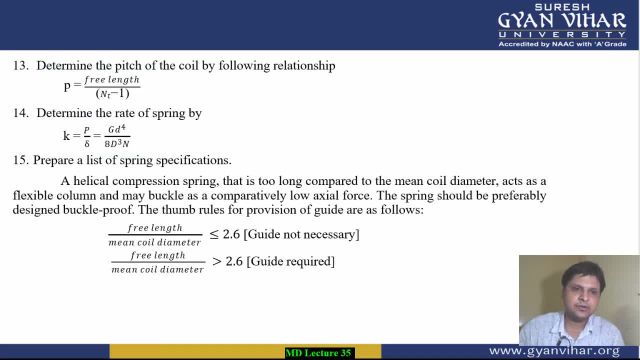 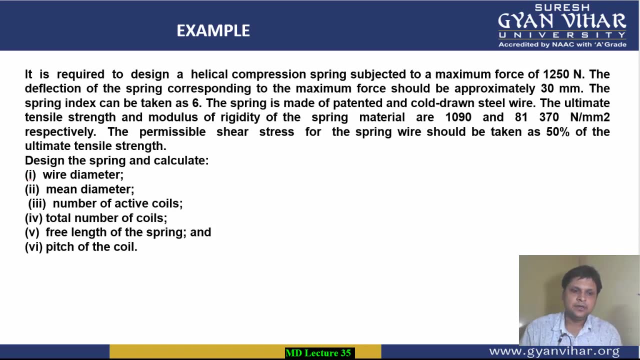 n. Alright, so these. this was the procedure which I taught to you in the previous lecture. Now, directly, we will solve the example. we will solve the numerical. Let's see what this numerical is saying. Let's read out this numerical. the numerical is saying that it is required to design a 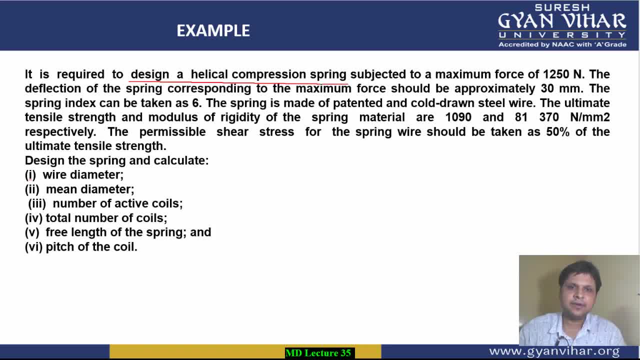 helical spring. So, basically, we are going to design a helical compression spring and it is subjected to maximum force of 1250 Newton. this is the maximum force means this has. this is the value of p. this is the value of p. then, after the deflection of the spring, corresponding to: 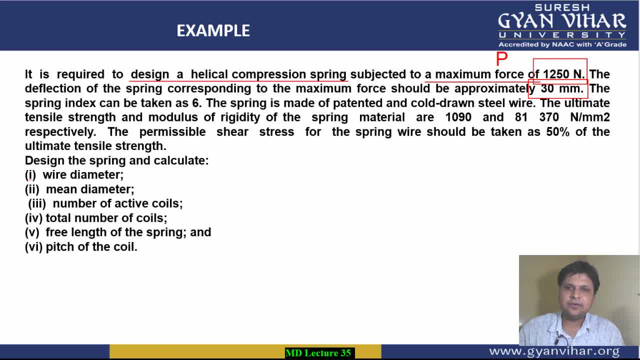 maximum force. Okay, This is also given to us. This is the value of deflection of the spring. So the maximum deflection means del value. they have given to us: 30,, 30 mm. The spring index can be taken as 6.. 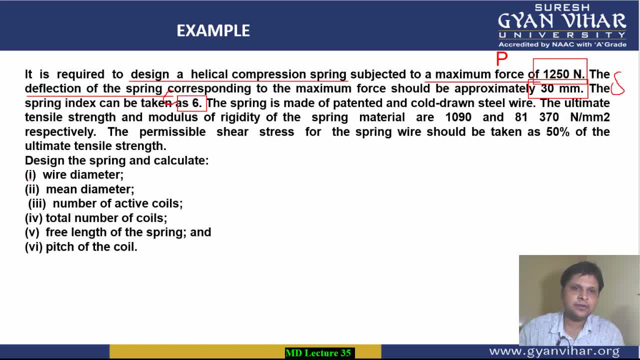 The value of spring index means capital C is also given to us. The spring is made of patented and cold drawn steel wire. This is the material from which the spring is made. The ultimate tensile strength and modulus of rigidity of the spring is also given. 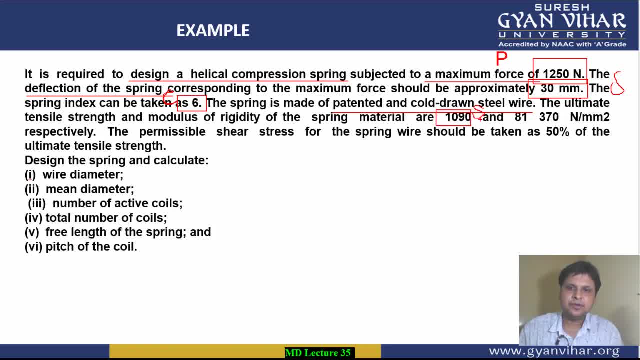 This is the ultimate tensile strength: 1090 Newton per mm square. This is the ultimate tensile strength. means this is sut and then 81370.. This is basically what this is, your value of modulus of rigidity. Alright, So we denote it by G in the formula. 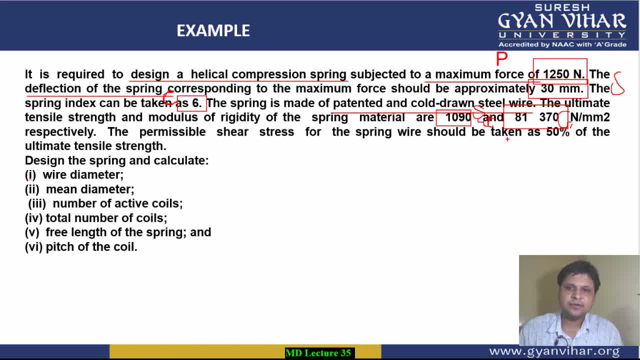 Then after, the permissible shear stress for a spring wire should be taken as 50% of the ultimate tensile strength. So the value of tau which we will take it will be 0.5. 50% means 0.2 into s? ut. All right, So this we are going to use the value. 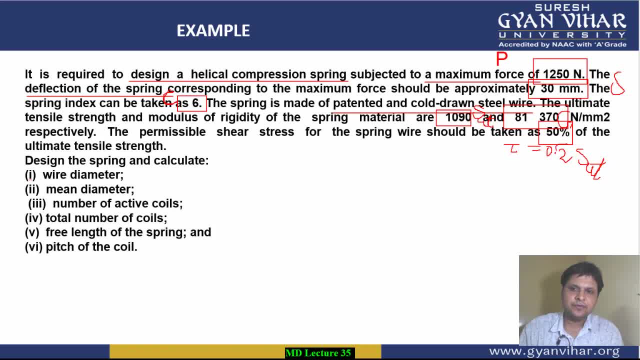 0.5. sorry, 50% means 0.5. this value we are going to pick. Then, after the, what are the values which we have to calculate in designing? we have to calculate the following things: First is the wire diameter, This means a small d. the coil diameter, this means capital D. 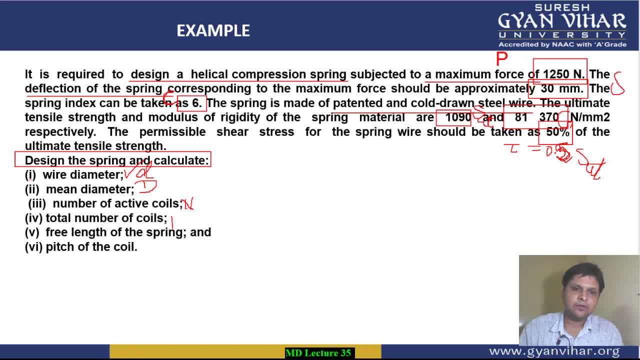 the number of active coils means capital, and then total number of coils means we write it by NT, then free length of the spring: free length of the spring and solid length of the spring. So whatever is the subscript you want to use, s, F, L, F, free length. All right then. 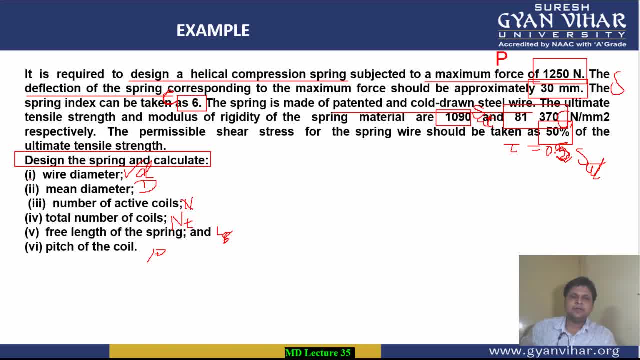 pitch of the coil. These are the values which we have to calculate, to calculate in this numerical. So, as we all know, we will start with the load stress equation and through load stress equation we can calculate these two values. These two values can be: 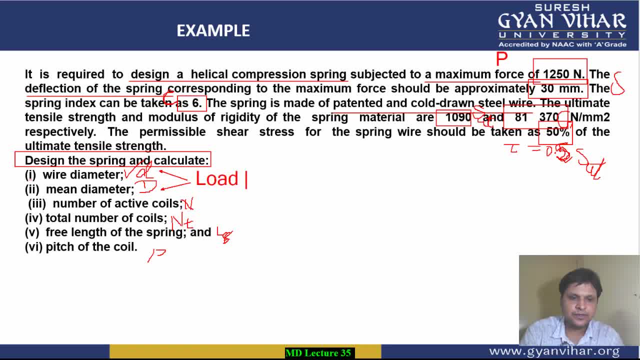 calculated by load stress equation. load stress equation. Alright, Then after what we will do for the number of active coils we are going to use the load, load deflection equation. load deflection equation: The number of active coils we are going to calculate by: 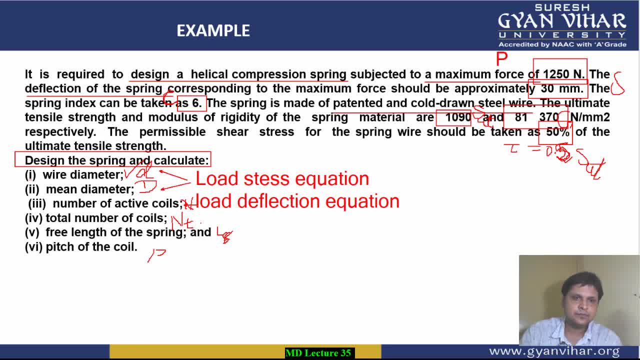 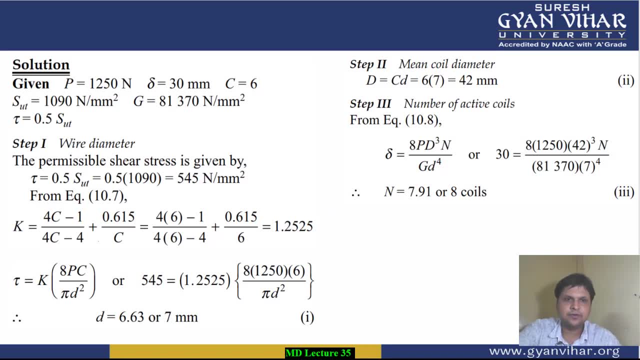 load deflection equation. Alright, then, after the following things which are remaining, they can also be calculated by the simple formulas. So let us, let us start See students. first of all, whatever values are given in the numerical, we have listed those values. These are the values: load is given to us: 1250 Newton, deflection 30 mm, then spring index. 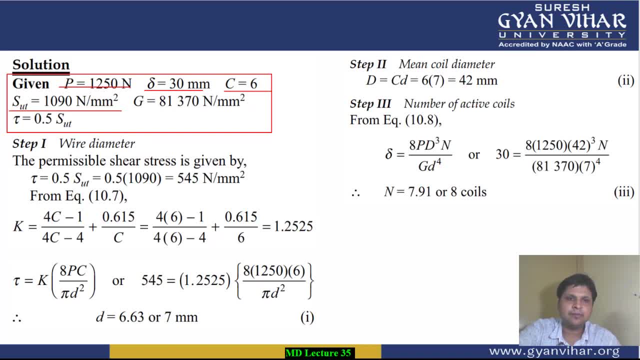 C. ultimate tensile strength value: 1090 Newton per square, modulus of radii: tg 8137 zero. this means that a material which is your steel, then the relation between the ultimate tensile strength and permissible strength, shear stress tau, is equal to 0.5 SU2.. So this will be our first step to calculate the 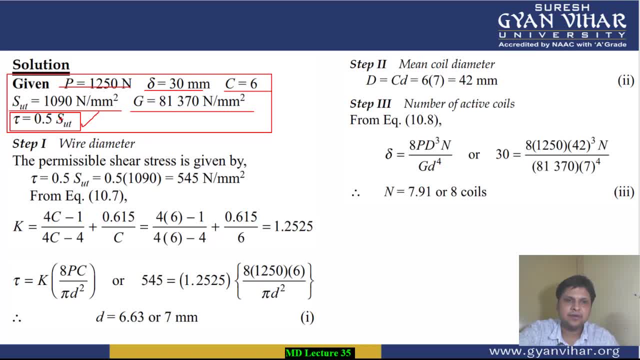 value of shear stress, because ultimate tensile strength value is given to us. So shear stress is equal to 0.5 of ultimate tensile strength. putting the value of ultimate tensile strength value given in the numerical, we can calculate the value of tau. alright, So tau value we. 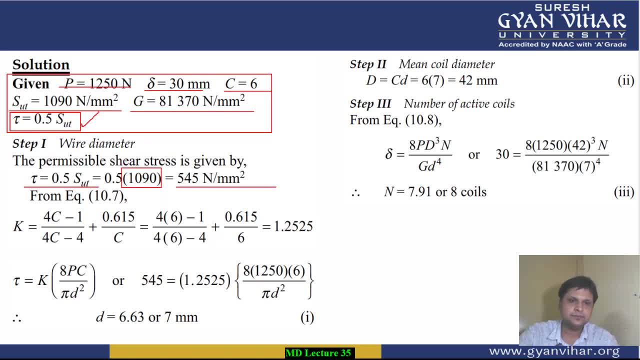 have calculated students, Then after wall factor, we will calculate How we will calculate the wall factor. The formula we already know: k is equal to 4c minus 1 upon 4c minus 4 plus 0.615 upon c. So this wall factor we will calculate, but for that we need the value. 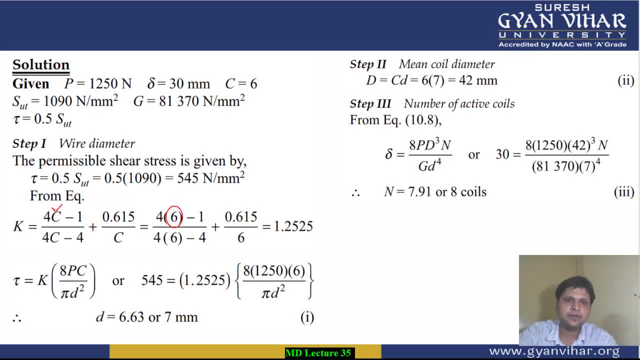 of spring index, and the spring index value is also given in us in the numerical. So this is the numerical. c is equal to 6.. This is the value of spring index. Directly using this value in this walls equation, walls factor equation, what we will get? We will get the. 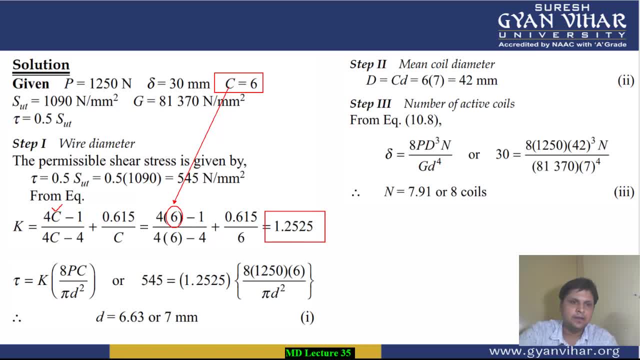 value of wall factor as 1.2525.. Now, using this wall factor equation, wall factor value in the load stress equation, which says that tau is equal to k into 8pc upon pi d square, We have simplified that equation. We have used the spring index, So we have used the 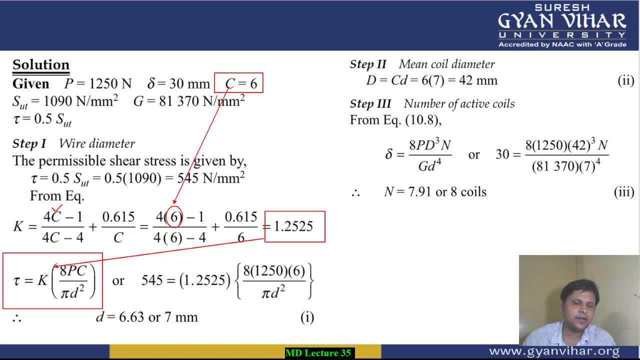 spring index, because we are having the value of spring index Tau is equal to k into 8pc upon pi d cube. Now if we put the value of spring index, load is also given to us- Then everything- k, we have calculated tau, we have also calculated here 545.. All the values are: 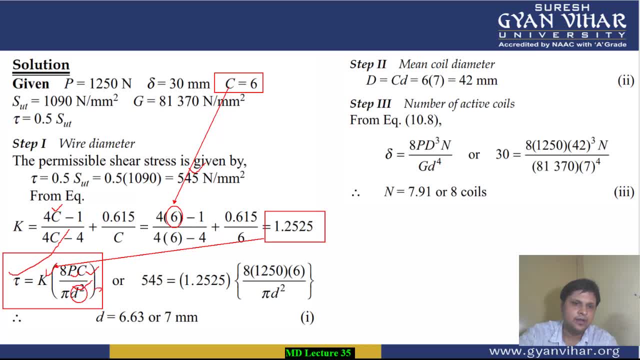 given, except the wire diameter, except the wire diameter. this So this is the unknown. So from the equation we can calculate the value of this unknown d. Alright, this unknown d can be calculated, Small d. if you will calculate you will find it as equal to 6.63. or if you round off, 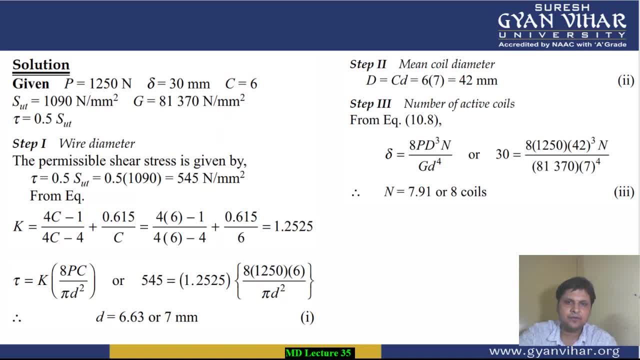 it will become equal to 7 mm. It will become equal to 7 mm. Alright, Now, if you have calculated the, if we have calculated the value of wire diameter, this means that we can calculate the value of coil diameter. How we will calculate the value of coil diameter: See spring index. 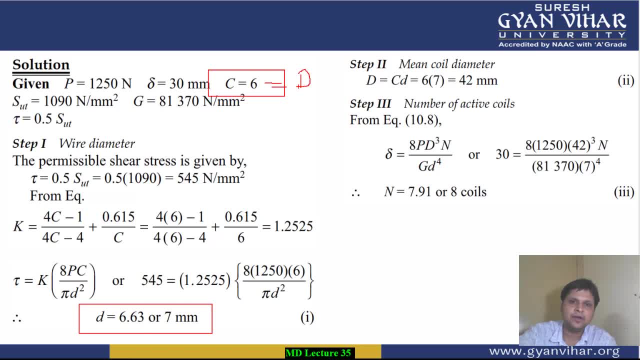 value we already have. and spring index is basically what It is, the ratio of coil diameter upon the wire diameter. So if c is there, small d you have calculated, then capital D will be equal to c into d. c into d means 6 into 7 means it is equal to 42. So this: 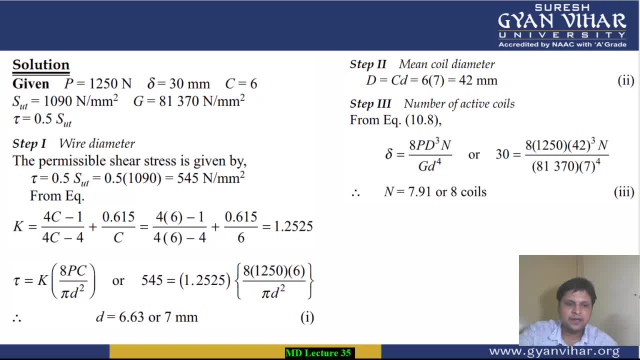 is the mean coil diameter. Alright, Then, after the next step, we have calculated the wire diameter and the mean coil diameter. Next step will be to calculate the number of active coils. So how we will calculate the number of active coils? As I have already told to you that 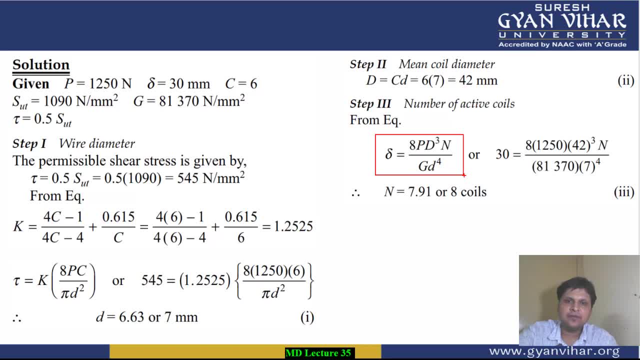 load deflection equation will fetch us this value. So this load deflection equation has got all the all the notations which we already have. Capital D: we have already calculated. Modulus of rigidity is given in the numerical, Then after load is also given in the numerical. 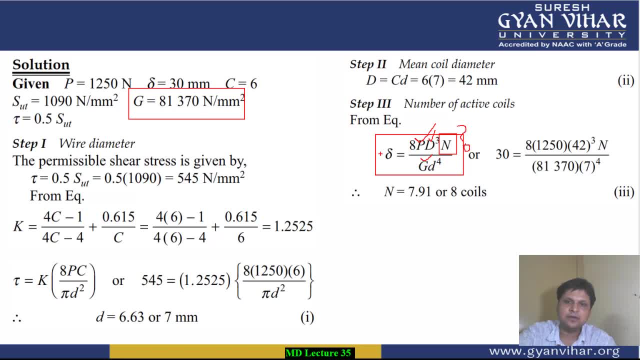 and number of active coils is the unknown which we have to calculate. All the other values are given to us, Using all the values like load 1250,, water diameter 42, mm. Then we have also modulus of rigidity 8370.. Putting all those values, small diameter means that the wire diameter. 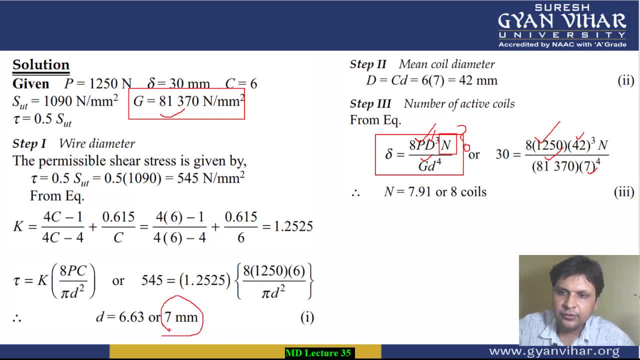 is 7 mm. That is also we have calculated here. So using these all values you students can calculate. from this relation to load deflection equation we can calculate the value of number of coils. number of coils are coming in decimal. We cannot have a coil in decimal because always 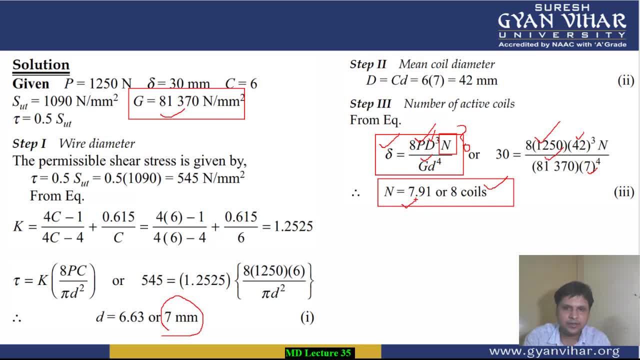 the number of coils. it should be in whole number. So this means 7.9. we will directly round off it and consider it as equal to 8 coils. Now, if 8 coils is the answer, not 7.9, if you consider it, if you round off it and taken as 8 coils, So total number of coils: 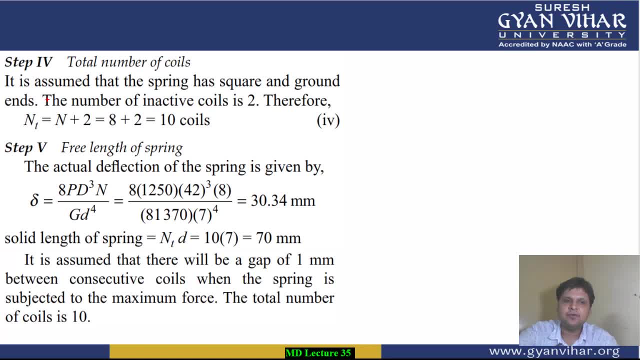 will be equal to how much? See now the total number of coils. as I have told to you in my previous video lectures that it depends on the type of style of end, that how much will be the total number of coils If the style of end is square and ground, if the style of 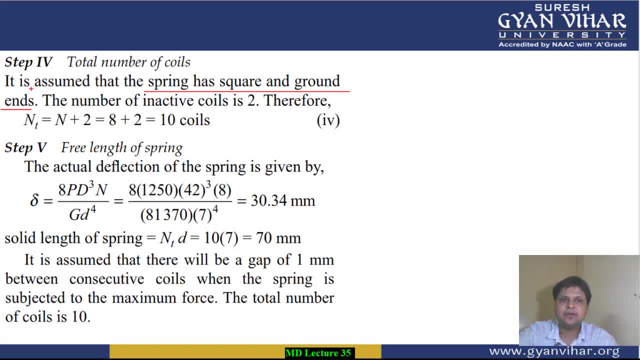 the end is square and ground. since it is not given in the question, So we are assuming it. we are assuming it that the spring has square and ground ends. This means that if the square and ground ends are there, Then in the spring, then directly, the number of inactive coils in such a style is your. 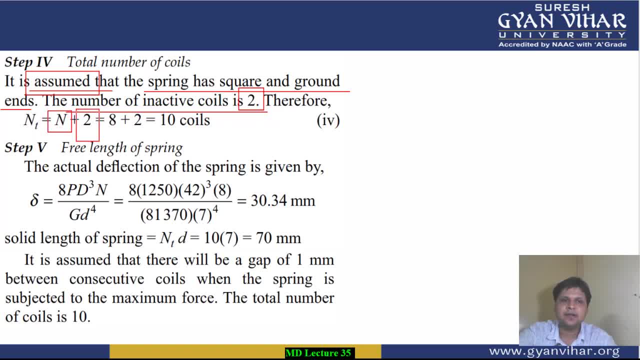 2.. So the total number of coils becomes active number of coils plus inactive number of coils. inactive number of coils: it is 2.. So n plus 2 will be give you the total number of coils. active coils, 8, inactive coils, 2. total will be equal to 8 plus 2. that is 10. alright, Then. 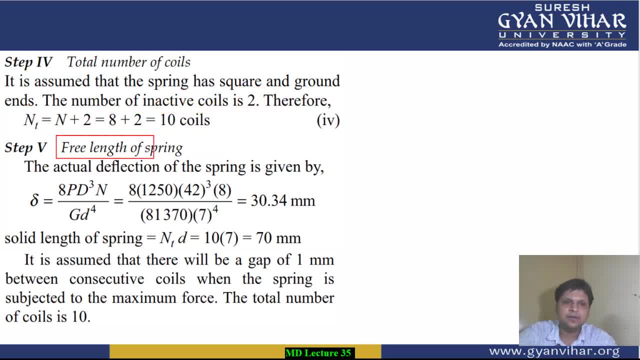 after, after the calculation of total number of coils, we are going to calculate the free length of the spring. Now for calculating the free length of the spring, what we will do. we have already seen the load deflection equation, which says that del is equal to deflection. 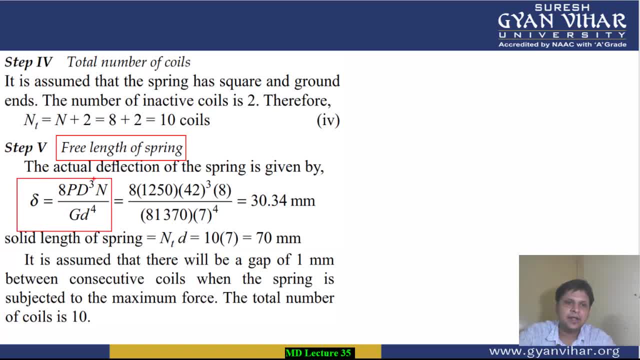 is equal to 8 Pdq n upon Gd to the power 4.. Here n value. which value of n we will take? we will take the value which we have calculated, that is, 8.. So, putting this 8 here, putting this 8 here, what we will get? We will get the value of actual deflection. alright, Actual. 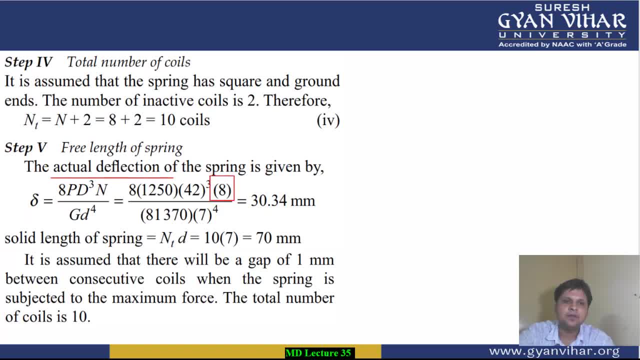 means: after designing, you have calculated a value of number of coils as 8.. So we will use this particular value in the deflection equation and we will calculate the value from the formula, the value from the formula which we have calculated. now this is the actual deflection. 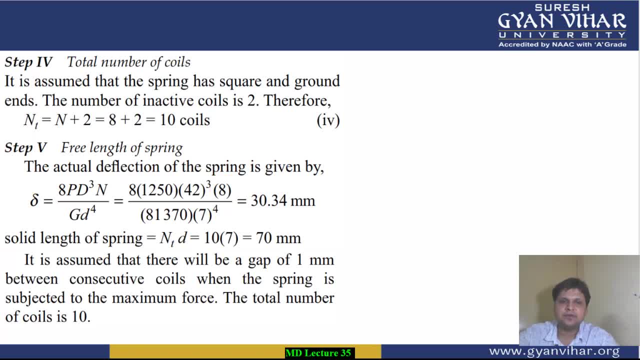 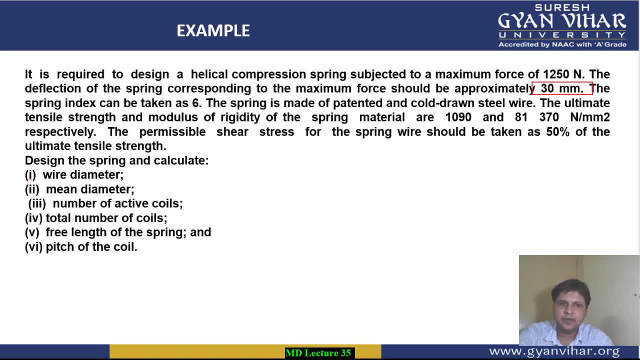 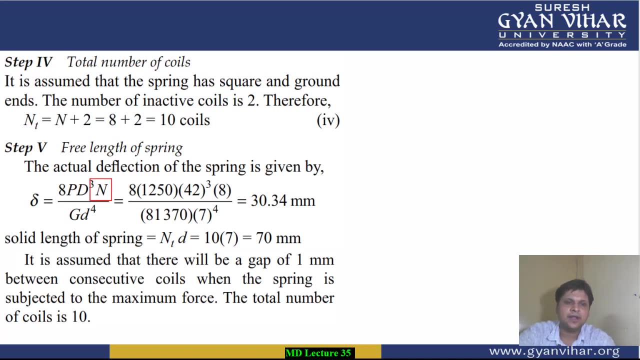 of the spring. This is what this is: the actual deflection of the spring, Though in the numerical the value of deflection was given to us as 30 mm. But actual deflection means that even if you have calculated the value of, if you have calculated the value of this n number of active, 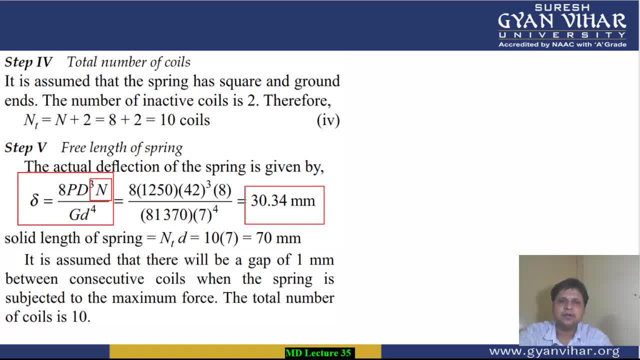 coils. So why not use this load deflection equation and calculate the value of deflection? So you can see in the numerical, the value given of deflection is 30 and the value which we have calculated, calculating by this formula, is 30.34.. So this is exact value. 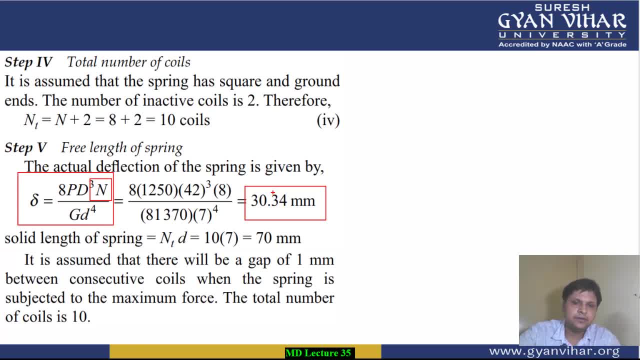 Now the solid length of the spring. how we will calculate Solid length, as I have already told to you while I am explaining you the different length of the spring- compressed length, solid length and the free length- At that time I have told you for calculating the solid length of the 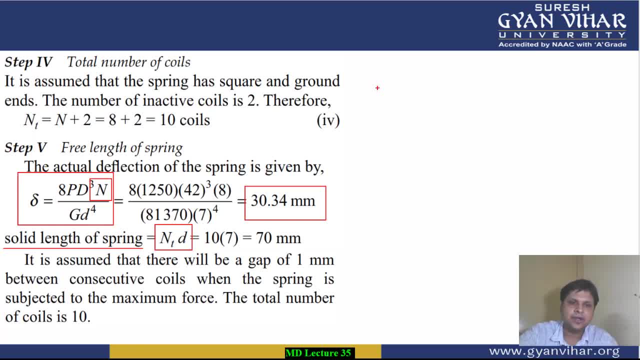 spring. for calculating the solid length of the spring, the formula is: your nt means total number of coils into wire diameter. So nt is the total number of coils into wire diameter. So nt is the nt into d. This is your solid length of the spring. Multiply these two values: total number of. 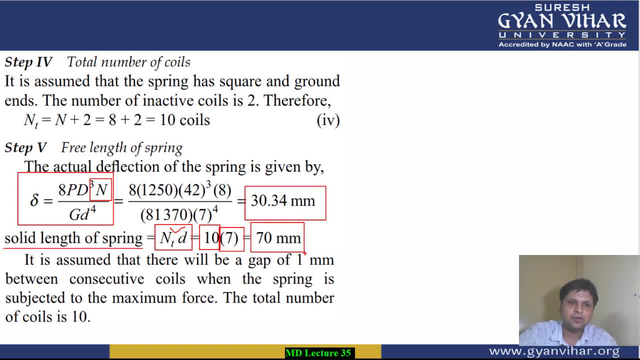 coils into wire diameter. This will give you the value of total solid length of the spring equal to 70 mm. Now it is assumed that there is a gap. Since there is no gap given to us, so we will have to assume something. See, assumption is important in the case of machine. 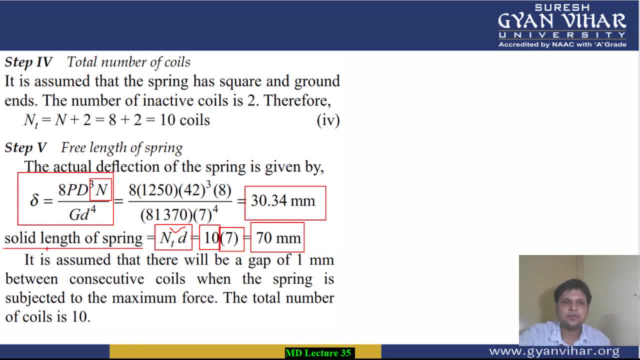 design subject, because sometimes whole of the designing we have to do and some values are missing. Those values which are missing, that values we can assume, but the assumptions is always practical Means. the values should be practical values. It should not be a value which 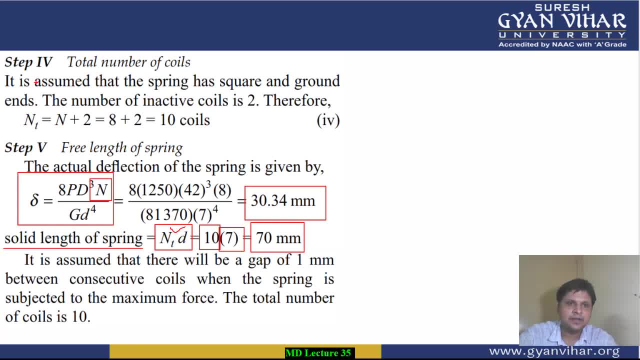 is not at all possible. Alright, see here, like in the case of style of end, we have assumed the style of end as square end, ground end. Similarly, here for gap between the coils, we have assumed that 1 mm is the gap between the two conservative coils. Now, if there is 1 mm gap between the two, 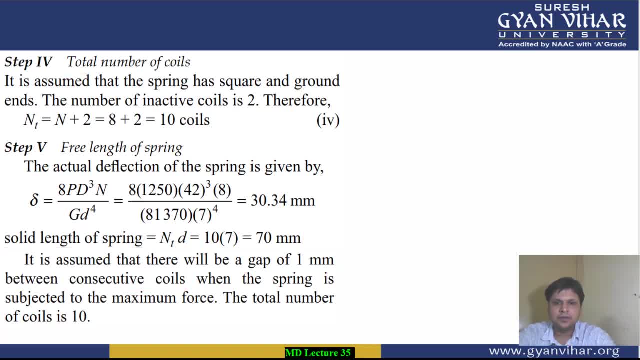 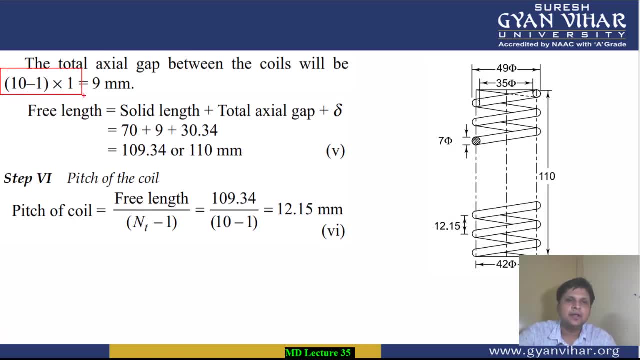 conservative coils and the total number of coils is 10, then how conclusion we can take out Nt minus 1- means total number of coils minus 1- into gap between two adjacent coils. This will give you the total axial gap. So how we are calculating the total axial gap. Total axial gap. 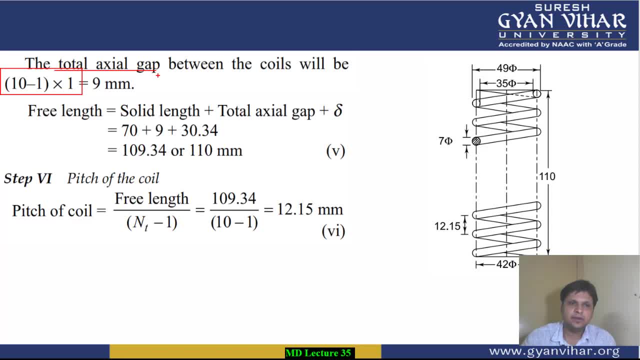 is equal to total number of coils minus 1 into the gap between adjacent coils, That is equal to 9 mm. So, finally, free length from this. finally, free length is equal to solid length plus total axial gap, plus del. This will give you the value. 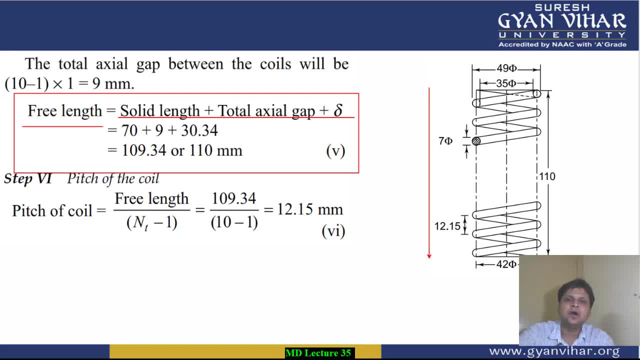 of free length: Alright, free length means complete length from here to here. So how you can get: If you will add the solid length, alright, plus the gap and plus the deflection, By adding all these three values you can get the free length. So free length will be 70,. solid length Axial. 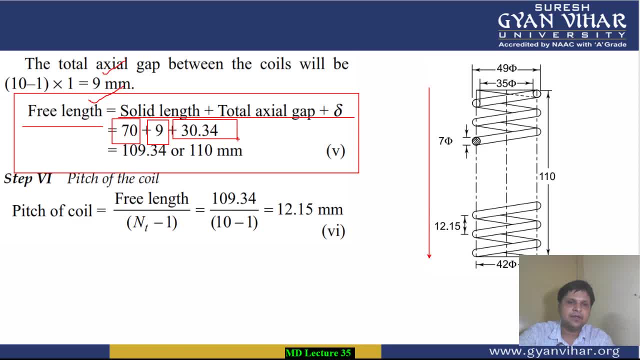 gap is your 9, which we have calculated here, And the deflection which we have calculated here. the actual deflection which we have calculated by the formula, is 30.34.. Adding these three values we will get the value of free length. So the free length value is 1, 1,, 0 mm, 110 mm. We have. 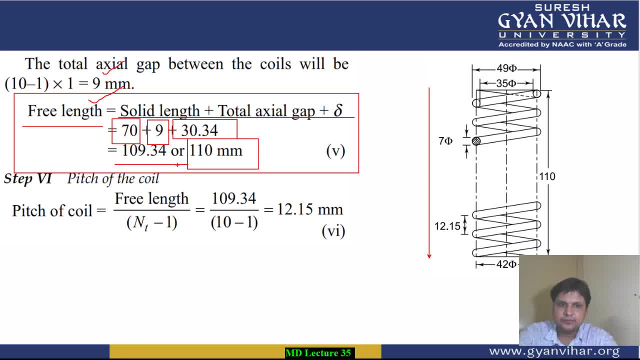 rounded off this 109.34 value. Again. the next step: the calculation of pitch of the coil. How we will calculate the pitch of the coil, The formula I have already told to you: pitch of the coil is calculated by free length upon Nt minus 1 into gap between two adjacent coils. So 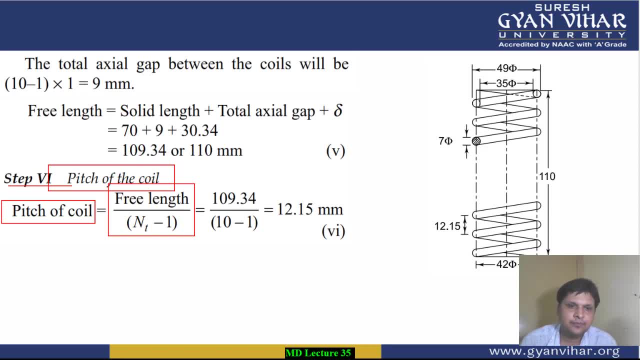 the value of pitch of the coil is 1 minus 1.. This provides you the value of pitch of the coil. Alright, so the free length we have already calculated in the previous step. in this step It was equal to 109.34.. Why not to take this actual value? So 109.34 we have taken, and 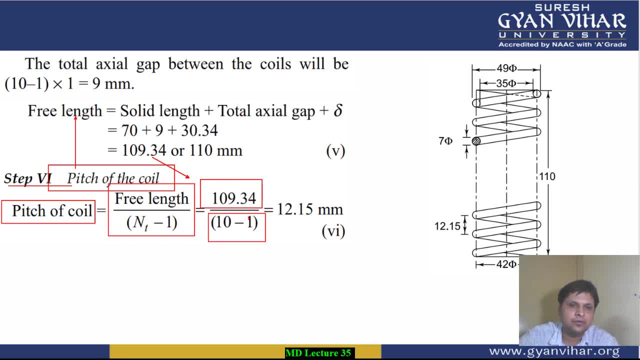 divided by Nt, is your 10 minus 1.. This will give you the value 9.. So 109.34 divided by 9, this will give you the value 12.15 mm. This is basically what. this is the pitch we have. 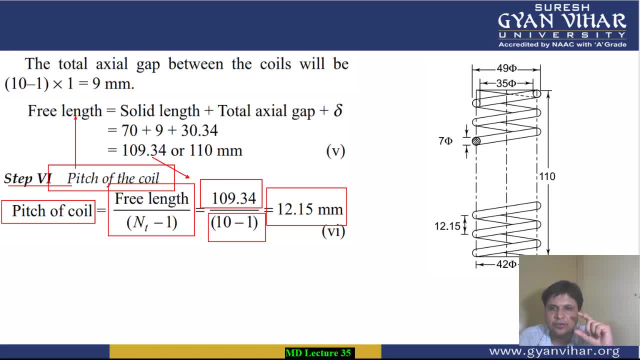 calculated Alright pitch is the distance between two adjacent points on the spring, on the adjacent coil of the spring. Distance between two, distance between two same positions of the coils of the two adjacent coils. Alright means one point if you consider here somewhere here. So 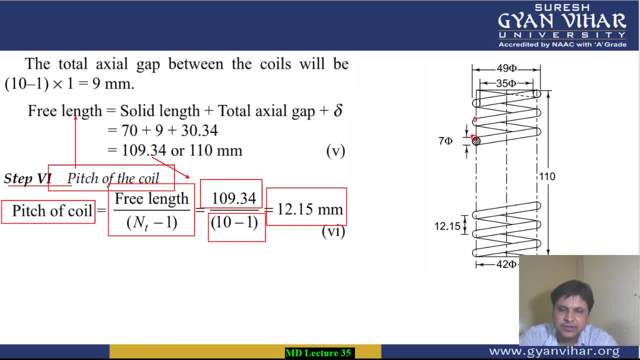 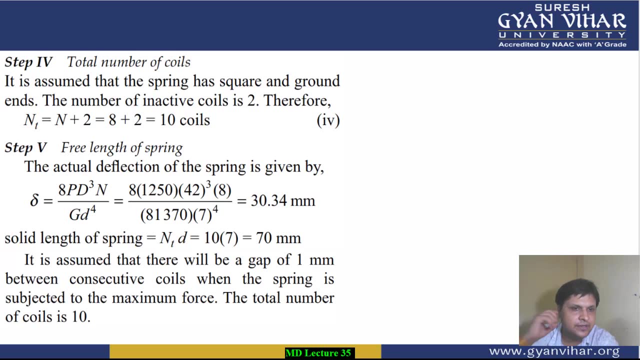 the same corresponding point on the adjacent coil, the distance between these two points. this will give you the value of pitch. Alright, so pitch, we have calculated 12.5.. What else is required to be calculated? Nothing, We have calculated everything in this numerical. So this was the whole sole numerical which we 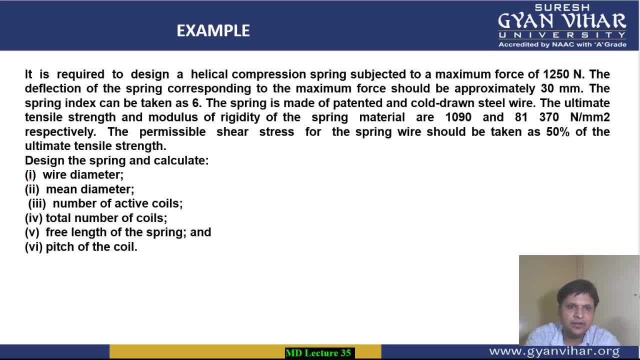 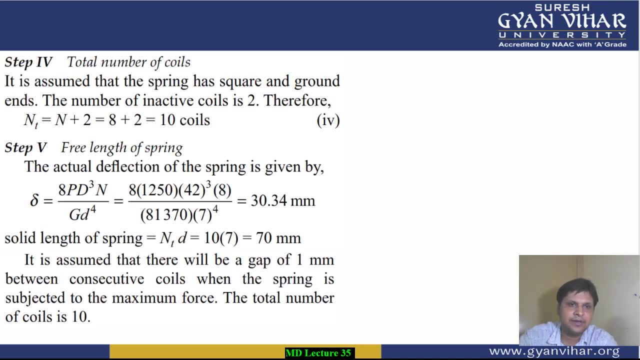 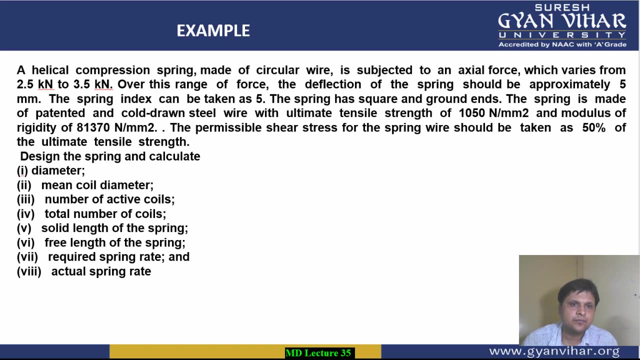 have solved. I hope you have understood, you have grasped the idea of designing of helical spring. One more numerical we will do and this will provide us a solidity in solving the design of spring positions. So let us see The next numerical. So this is the next question, student, Let us read out the question and see. 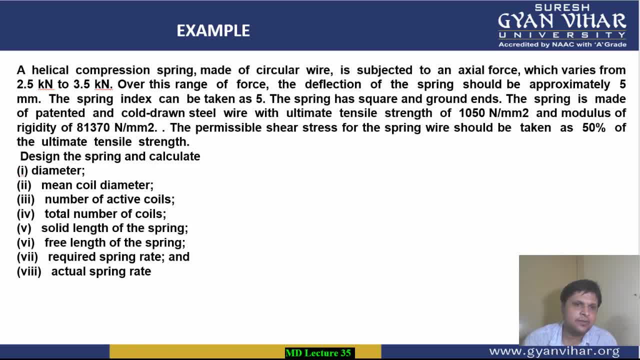 what values are given. So in the numerical it is saying that a helical circular, a helical compression spring made of circular wire. alright, the cross section is circular, It is subjected to force which varies from 2.5 kilo Newton to 3.5 kilo Newton. So this value they have given. 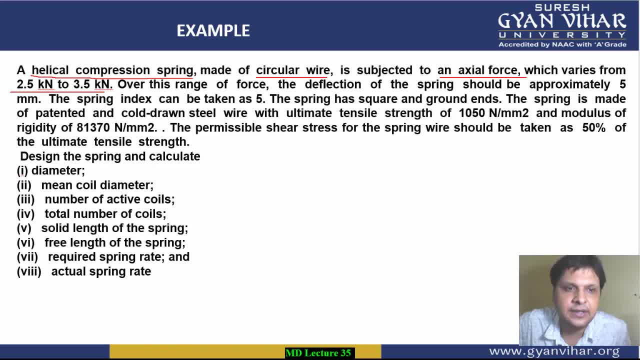 they have not given you the exact value of load. they have said that the load is varying between 2.5 to 3.5 kilo Newton. over this range of force, the deflection of the spring should be approximately 5 mm deflection. also, they have given to you, in this range, Alright deflection. 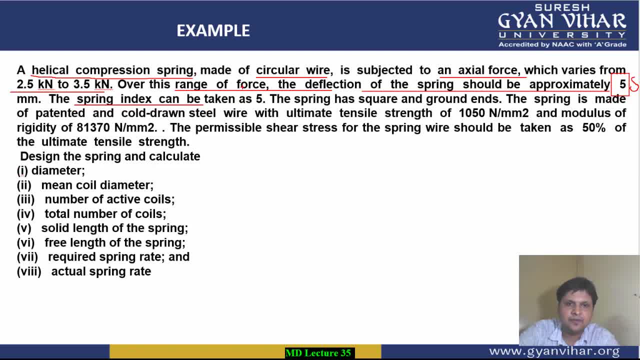 is given to you again. moving further, spring index can be taken as 5,. 5 is your spring index, which is denoted by capital C. The spring has square and ground ends. So this is the type of spring ends: square and ground ends. The spring is made of patented and cold drawn. 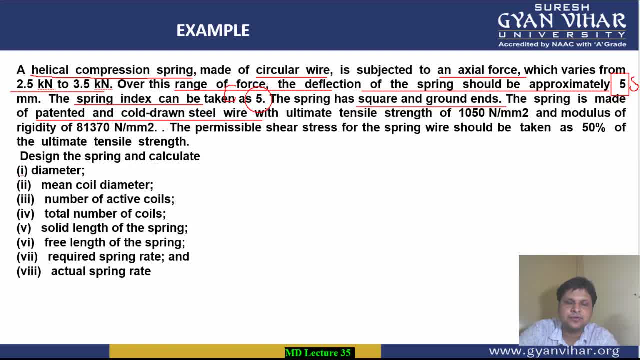 steel wire: Alright, this is the material that is used to make the wire. patented and cold drawn steel wire, The style of end in this previous line. this particular value will provide as the value of relation between the total number of coils and the number of active coils, So NT total. 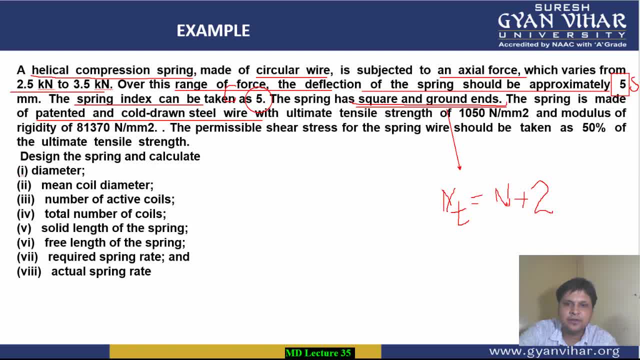 number of coils. if we have calculated the value of active coils, then total number of coils will be given by N, number of active coils plus 2.. This is in the case of square and ground ends. So this value we will take. moving further, the spring is made of 5, 5,. 5, 3, 4 and ground ends. The spring can be taken as any particular material of different types of same kind because these are the unique pieces-. às a caution, because the explainings of the emotion coming happened that cut by section are generally affect the. 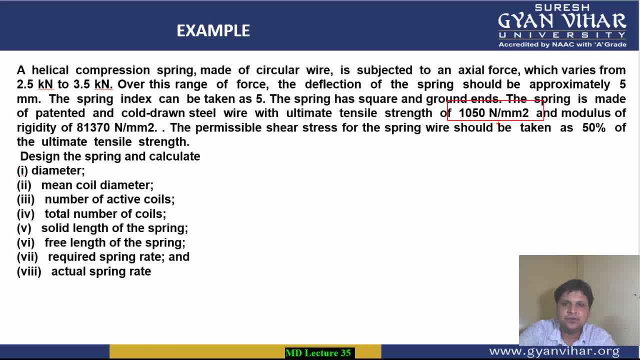 members of the own tissue, because machine evermon, flourğl, bymates. We know that in all types of materials there are other processes similar to your life that are made from all kinds of materials, that are made of different kind of materials unlike a few olacak. let us say you used to make ligament or a charcoal oil, which? 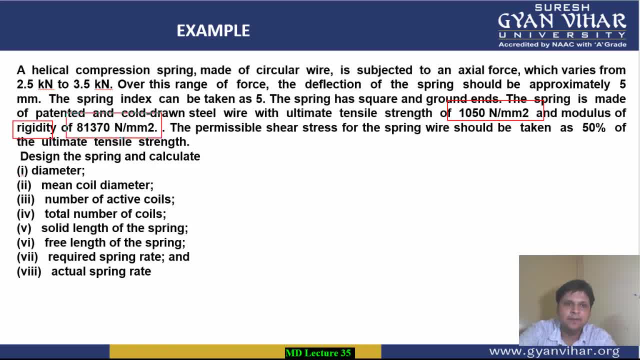 is been made of. there are different types of material here: bolts, mus, Zelda saying that they are made of this, This we have already read the lines. The ultimate tensile strength value is given, 1050 newton per mm square, and modulus of riginity is given to us as 81370 Newton per mm square means this is the value of capital. 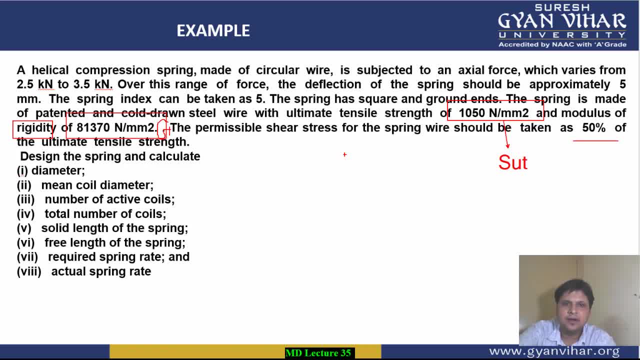 the spring wire should be taken as 50% of the ultimate tensile strength. So the same line we have used in the previous numerical, also tau. we have to take 0.5 into ultimate tensile strength, SUT. Alright, Now what values we have to calculate here Again. first, 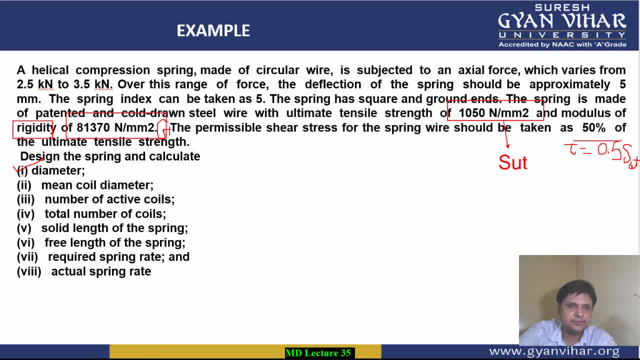 is your wire diameter. second is your coil diameter. third, number of active coils. So this means that small d, capital D, Based on this spring index, we are going to calculate the number of active coils. capital N- Total number of coils means NT. we are going to 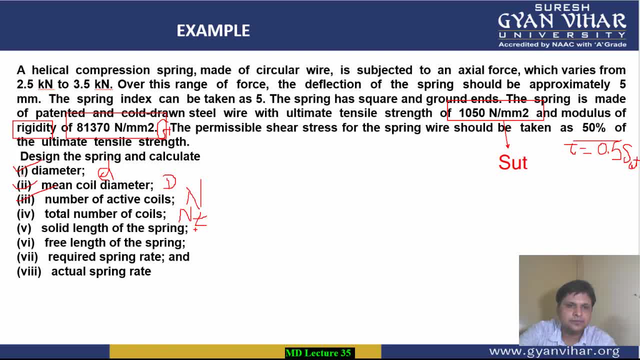 calculate. Then, after solid length of the spring, three type of length: solid length, free length. These two length of the spring we will calculate and then, after required spring rate, we will calculate the spring rate, Alright, And then at last, actual spring rate. So, two type of spring. 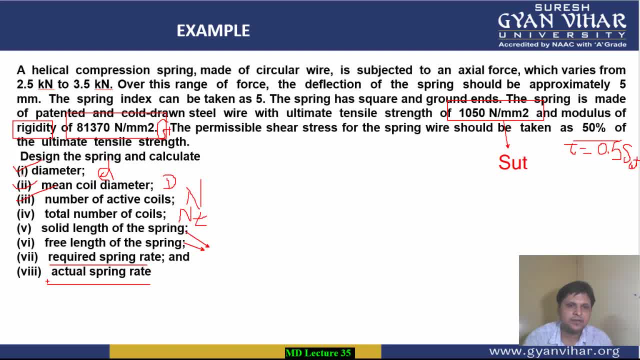 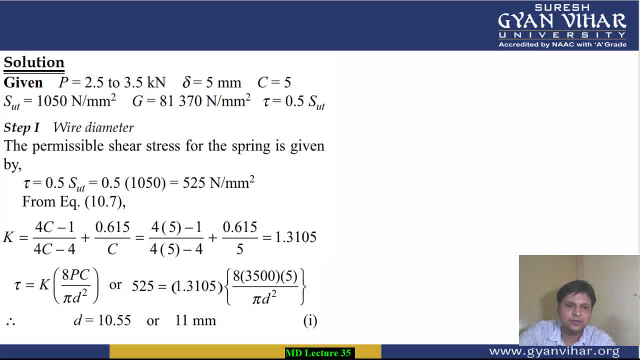 rate we have to calculate. One is the required spring rate and then after the actual spring rate. So let us see move into the solution now. So first of all we will list out all the values which are given in the numerical. 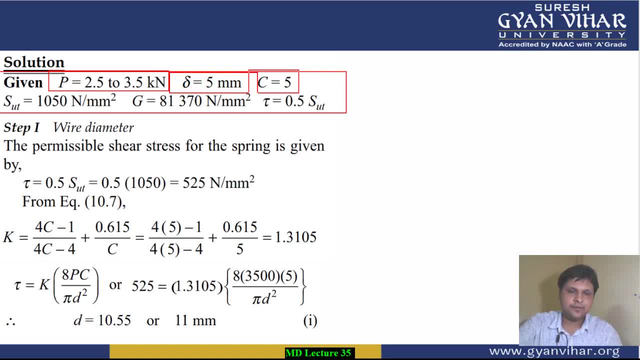 These are the values Load we have been given as VDES. Then, after deflection, the spring index, ultimate tensile strength modulus of relative g, and then tau value is also given to us. So first step is to calculate the wire diameter, The permissible shear stress for 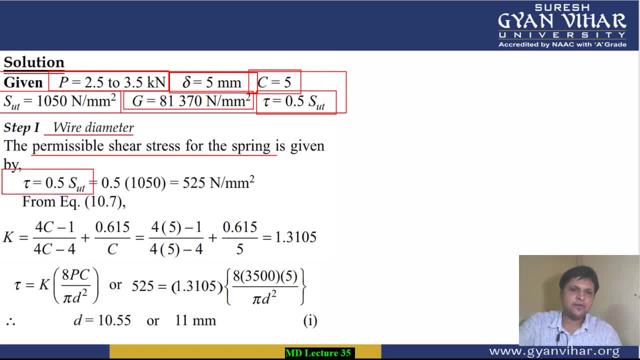 the spring, is given to us as tau da and tau dao Andowed by the pressure flow rate for that stretch value, your soient length or length of your umm fruits load of yourование's tau is equal to 0.5 of ultimate tensile strength. So this formula, we already know and it is 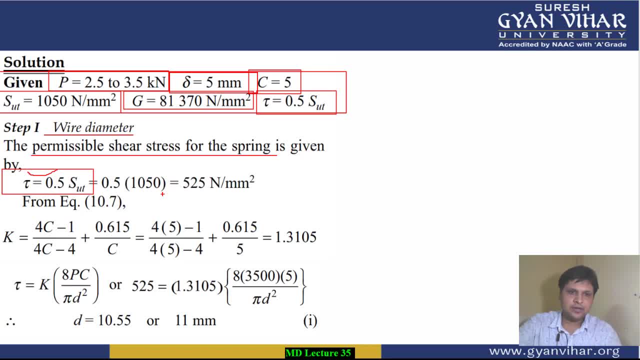 also given in the numerical also. So, using this particular formula, we can calculate the value first, value first important value, that is, the shear stress value, permissible shear stress value. Now, using this value, using this value, we can calculate the wall factor, wall factor relation. we already know All right and how we will calculate, only spring. 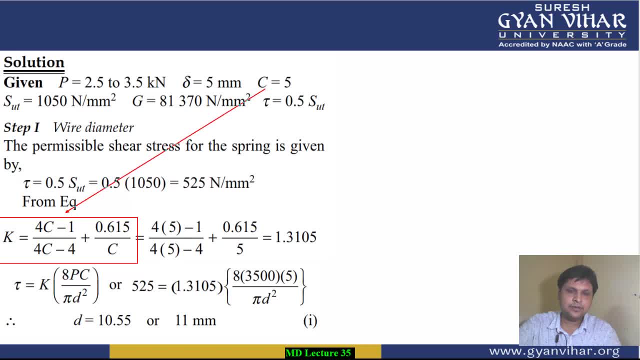 index value we need and spring index value given to us here. Using this value here, in this formula of wall factor, we can calculate the wall factor. It is 1.3105.. Then, after the shear stress value, tau is equal to k, into 8 PC upon pi d square, In this particular 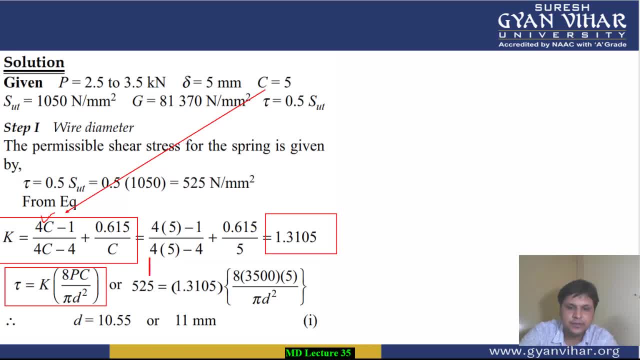 formula. this is basically the formula of load deflection. This is your load deflection, load stress Relation, this is your load stress relation. through this relation, two values can be calculated: one is the wire diameter and then, after after calculating it, we are going to calculate the. 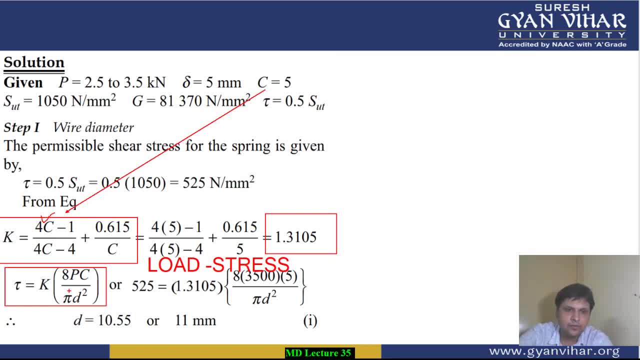 coil diameter, So wire diameter, that is your small d. we will calculate from this the values which are given to us in the question. is your spring index, then after that load that is acting and then after the wall factor we have calculated and the permissible stress shear, 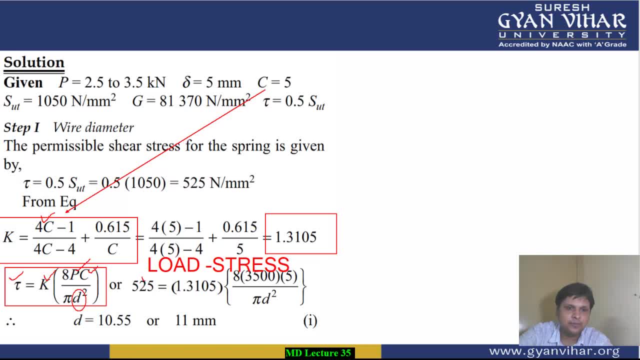 stress value also. we have calculated, Putting all these values alright. load value: one thing you should keep in mind: that may always in this equation the load which is taken in the maximum load- So don't get confused with this particular language- that the load is varying between 2.5 to 3.5 means that always. 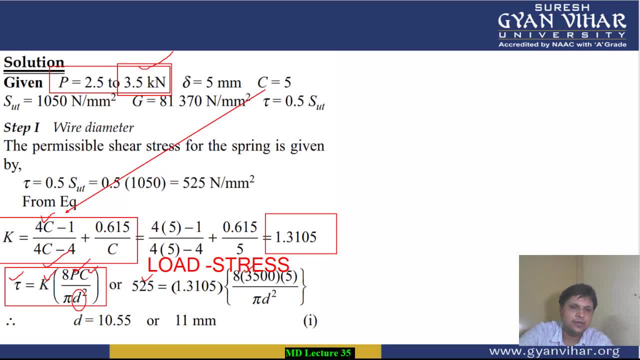 we will take a maximum value in this equation. the load value here in this equation, in this load stress equation, is the maximum value of load. So we will take in between 2.5 to 3.5.. What is the maximum value? Mattion values is 3.45.. So 2.5 is modêu value in this case. 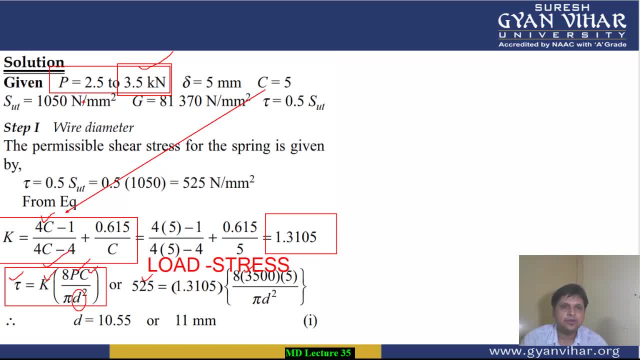 is the weld value as well. this value is less than or minus 0. we have to use our load value to calculate the load on T defined value. again, these values are used to calculate load value values in kilo. it is in kilo newton, so in newton we will say it is equal to 3500, 3500. so in the low. 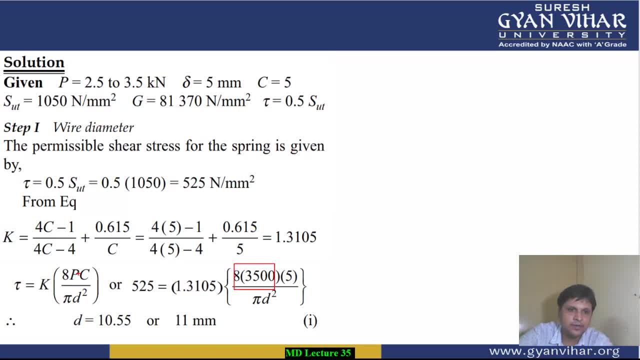 stress equation. we are going to put the value 3500 in the place of this p. all right, all other values are already known to us. then, on putting these values, we will get the value of wire diameter as equal to 10.55 mm. i hope you have understood till now. now, based on as we have done in the 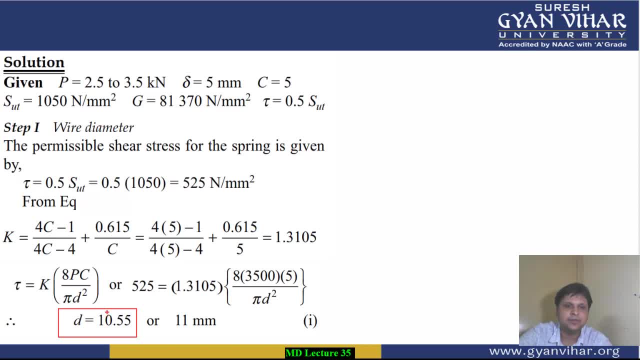 previous numerical, similarly here, also based on this wire diameter and based on this particular spring index, we are going to calculate from these two values. we are going to calculate the value of coil diameter how we all know that this particular value, this particular value of c, is ratio of what wire diameter, coil diameter divided by 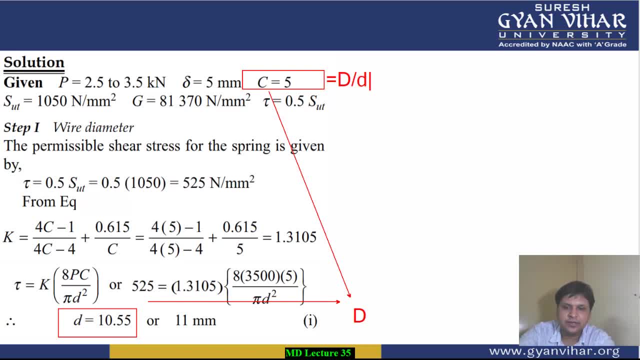 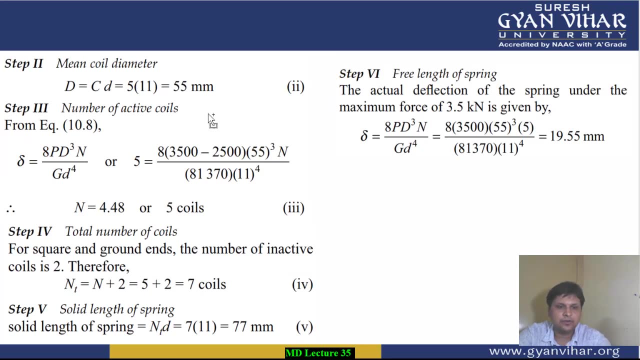 wire diameter. all right, so putting the value we can get capital d lord, capital D divided by a small d is equal to 11. And this is equal to five means capital D will be equal to five into 1155.. So, moving further into the solution, as you can see, 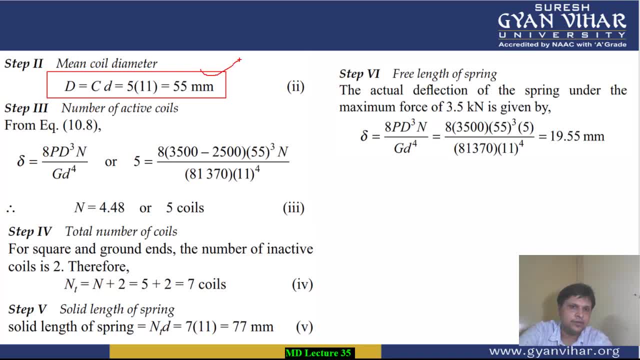 as I have told you, the value C into D will give you the value of mean coil diameter as 55.. Now the next step is to calculate the number of active coils. So the number of active coils, students, how we can calculate C, As I have already told you in the previous. 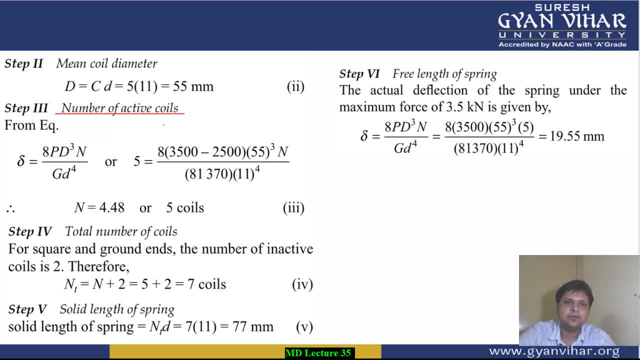 numerical and in the design procedure also, that the number of active coils is obtained by the load deflection equation. And this load deflection equation, deflection is given by 8 pd cube of n upon gd to the power 4.. So g is your modulus of rigidity, Its value: 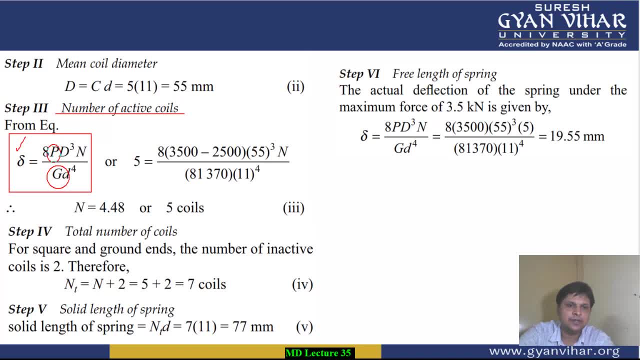 is given in the numerical Load. we will take the maximum here, in this equation, in the equation of load and deflection. Keep it in mind. the one thing, one twist that is there, is that here we will take the difference of the load, that is the. 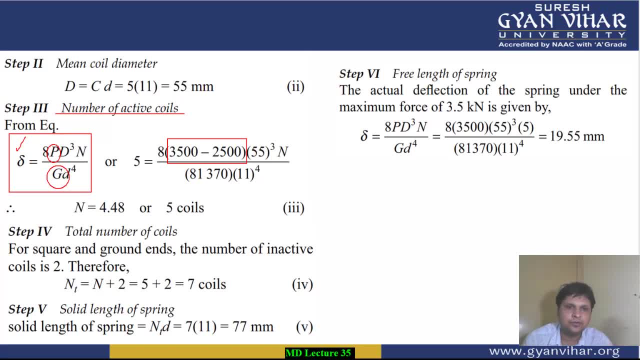 maximum load and the minimum load. So we will take the difference of these two values- Difference of the maximum load and the minimum load. we are going to take here in the load deflection equation, while in the case of stress load equation we have taken the maximum value. 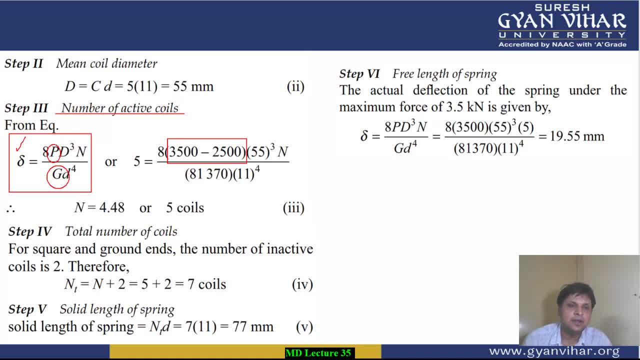 of load. Alright. so this you should keep in mind: that always, whenever such case is there that you have been given the value that the load is varying between two values, then always the difference of the values of the load you will take in the case of deflection. 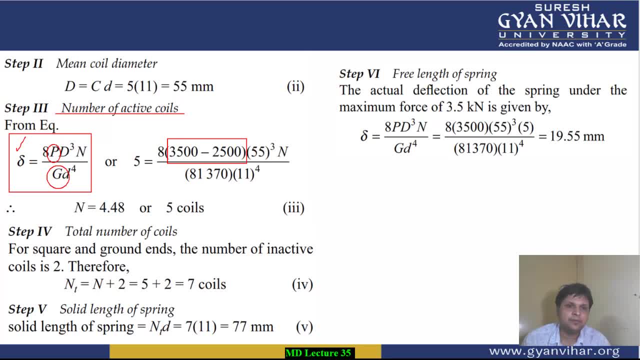 equation, while for stress equation you will use the maximum value. So this is the deflection equation for calculation of number of active coils, For in this equation we are going to put the value of p as difference of the values of maximum and minimum And capital. 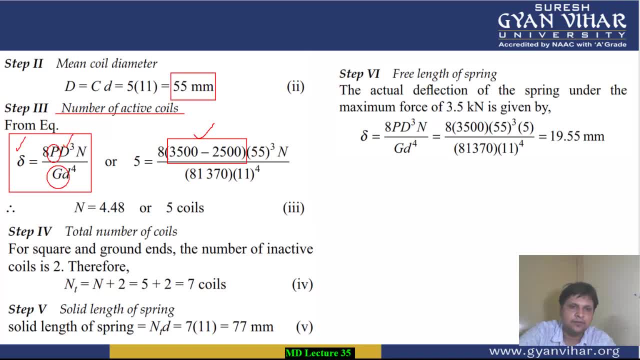 D is what Capital. D is the mean coil diameter: 55 mm already we have calculated. Then after g is given to us as 8133.5 mm. So this is the difference of the load you will take in the case of deflection equation, While in for stress equation you will use the maximum. 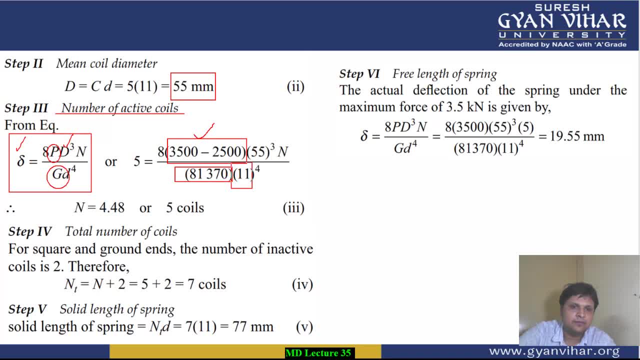 value of d70, modulus of rigidity of the material. Then small d is wire diameter is equal to 11.. So all the values are given to us. even the deflection value was given to us in the numerical. So based on it, we have calculated the value of. based on it, we have calculated. 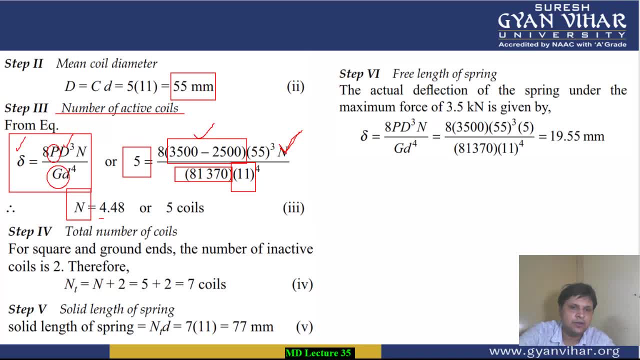 the value of the number of active coils. Number of active coils, we are getting 4.48.. So obviously coils can't be in decimal form. So we are rounding it off and we are taking the maximum value, that is, 5 coils. 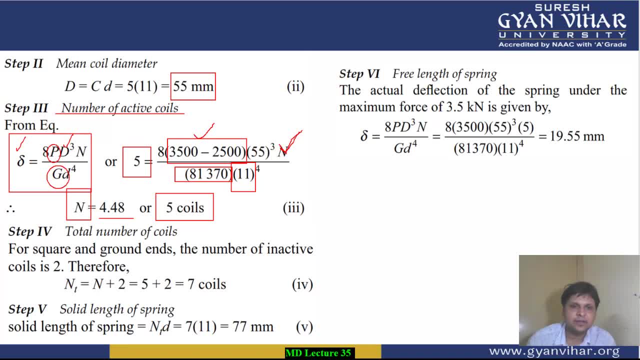 Now, always we take the larger value in designing. we don't take the smaller value, like for example here. there might be a thought in your mind that 4.48 will be round off to 4, but it is not like that. always the next larger value is taken. Therefore, we have taken the value. 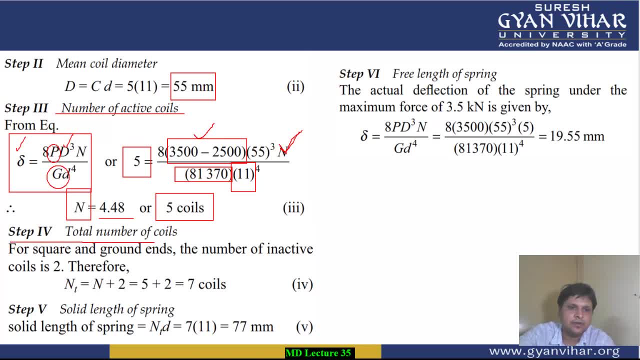 5.. Then, after the next step is total number of coils. step number 4, that is the total number of coils. How we will calculate. See, the coil has got square and ground ends. This is given in the numerical: If the coil has square and ground ends and the number of active coils. we all know that. 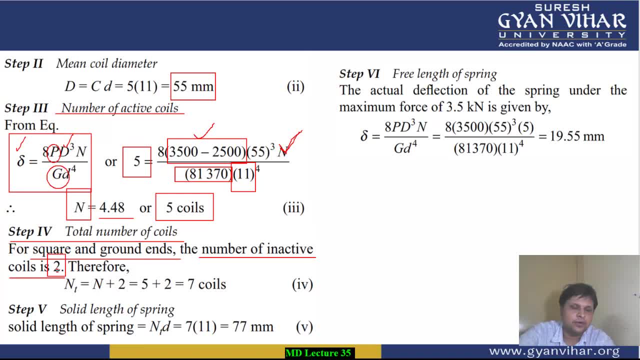 for square and ground end is equal to 2.. So for the total number of coils, we can calculate by adding these two with the number of active coils. Number of active coils we have already calculated equal to 5.. 5 plus 2, this will give you the value of number of total coils. 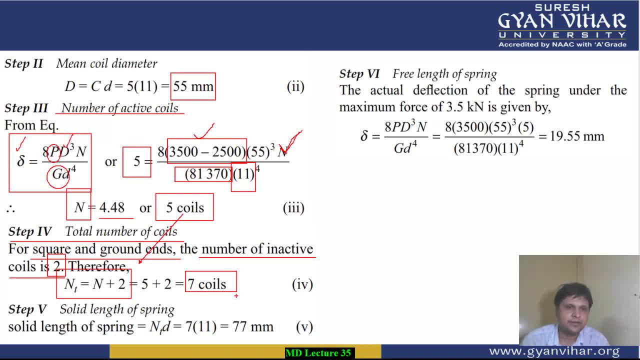 as equal to 7.. 7 coils. Alright, this is the total number of coils. Then, in the designing, what is the next step? We are going to calculate the solid length Based on this particular value of total number of coils. we can calculate the solid length. How we can calculate We. 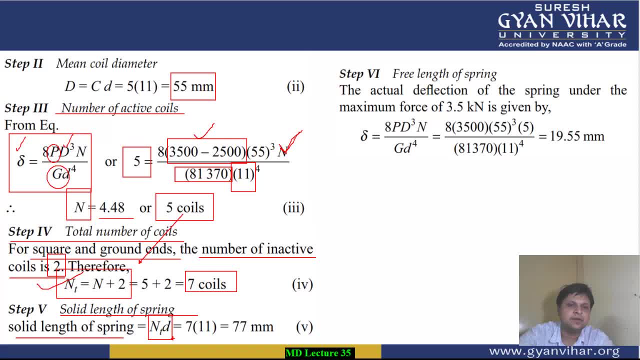 all know, solid length is given by multiplication of wire diameter with the total number of coils, So Nt into D, that is, 7 into 11.. This will give you the value equal to 77.. 77 is the solid length. Then, after students, we will calculate the total number of coils So Nt into D. that 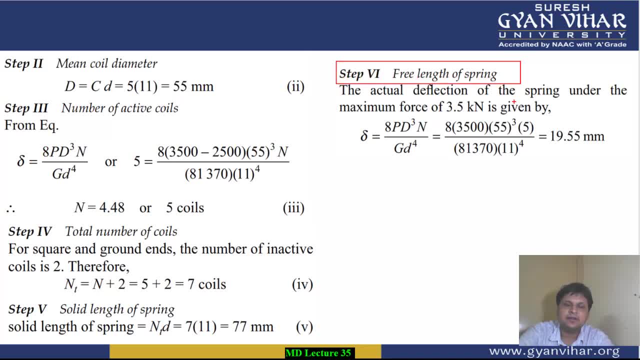 is 7 into 11.. Our next step will be to calculate the free length of the coil. And how we will calculate the free length. See, already I have told to you that free length can be calculated, but for that you will have to use the value of deflection And again you will have to. 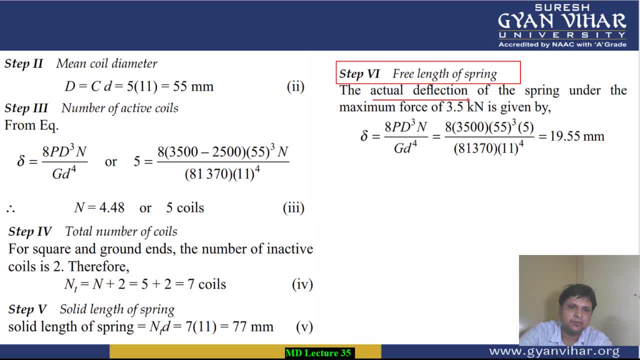 calculate actual deflection, Though you have got the value of deflection in the numerical, but that value you will not take here. That particular value of deflection, which is 5, you will not take here value in the calculation. For this particular value you will have to take actual value. So for actual value all 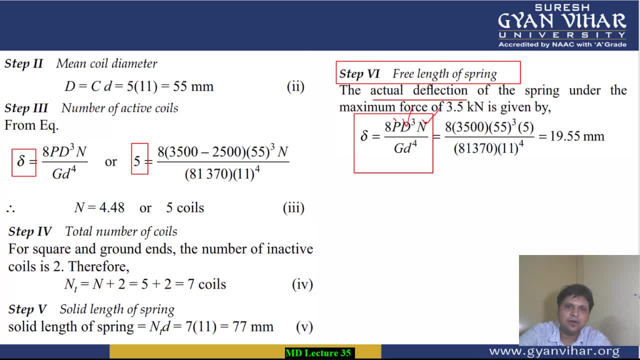 the values like number of active coils, wire diameter, coil diameter, load, all values you have in the load stress equation, in the load deflection equation. in fact, what we will do, this maximum value we will take of load For actual deflection, what you will have to do, 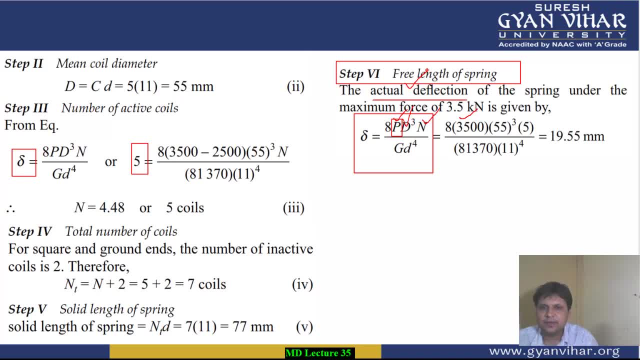 you will not have to take the difference of the values of the load, The maximum load value you will take. So the P capital P we are taking as the maximum value and it is equal to 3500. Because the load is in between 2.5 to 3.5 kilo Newton. So maximum value is 3.5 kilo Newton. that 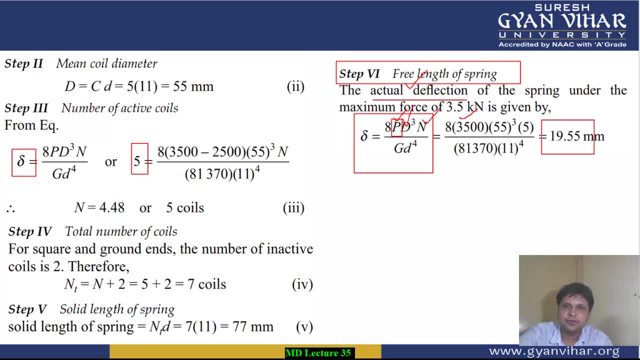 same value we are taking and putting in here in the equation. So by doing this, the value of deflection which we are getting is 19.55 mm. This is the deflection value which we are getting, actual deflection value. Now, this actual deflection value, why we are calculated? Because we have to calculate. 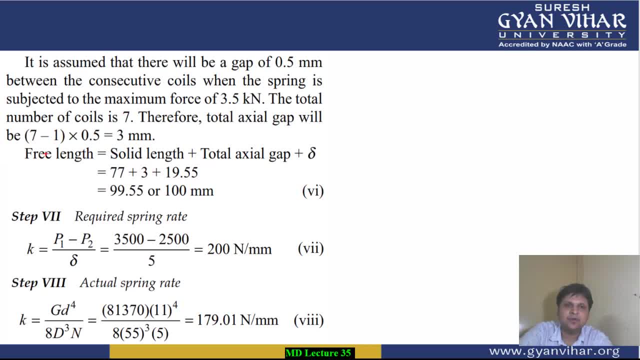 the total length and for that we have to calculate the gap, total axial gap. The total axial gap is only possible if we have the value of total number of coils. All right, total number of coils is 7.. Nt-1 means total number of coils minus 1 into gap between adjacent coils. It will give you the value of total lengthgi, from x comma of height to Gh. That is how you calculatelen is calculated Now, this actual deflection value. why we have to calculate? Because we have to calculate the total length And for that we have to calculate the total. 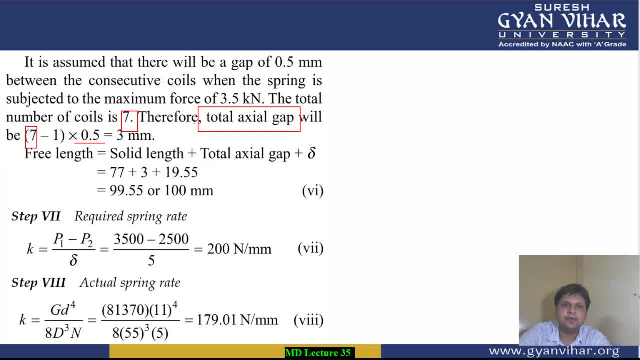 total axial gap. So total axial gap will be equal to what gap between adjacent coils is 0.5? we are assuming it is not given in the numerical. as I have already told you, we will have to assume some values which are not given in the numerical, like the gap it is not given. 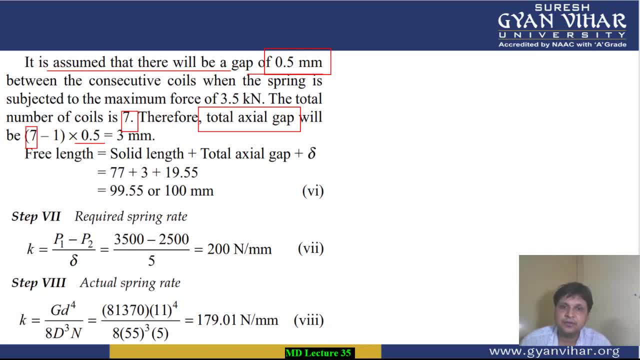 So we can take some, some value which is actually practically possible. 0.5 mm is the generally common gap which is taken between the two coils in the case of helical springs. So we have taken 0.5 mm Now doing this. 0.5 is the gap between two adjacent coils. Total number: 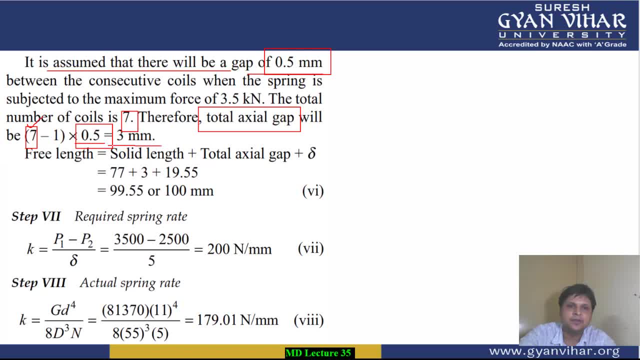 of coils is seven, So nt minus one into 0.5.. This will give you the total axial gap. On calculation, you will see that total axial gap is equal to 3 mm. It is equal to 3 mm, All right. Then after from this, from the total axial gap, 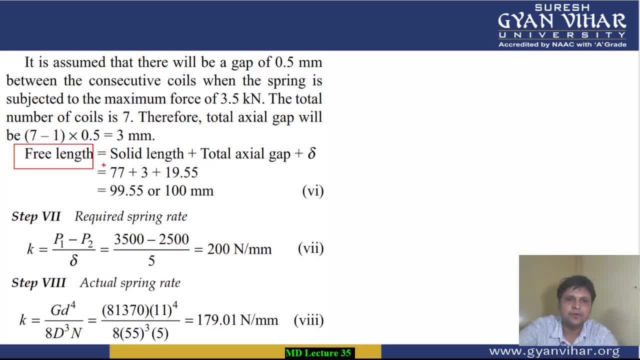 we will have to assume the total axial gap is equal to same as the gap between the two axial gap value. we can calculate the free length because we know the formula: free length is equal to solid length plus total axial gap, plus this particular value of actual deflection, Actual. 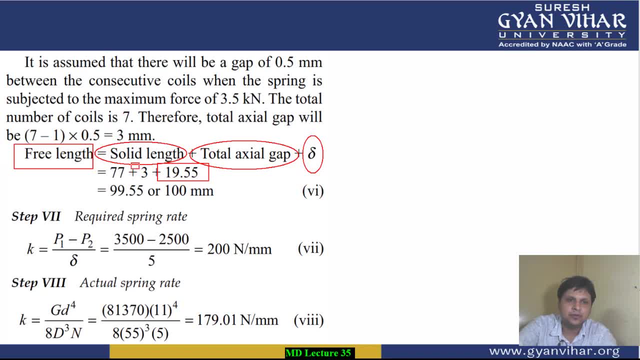 deflection we have calculated is equal to 19.. Total axial gap: here in the above step you can see 3 mm we have calculated. Solid length, which we have calculated is 77.. Finally, on adding these 3 values you will get 99.55 as the free length. So nearest hole number near to it is 100 mm. So 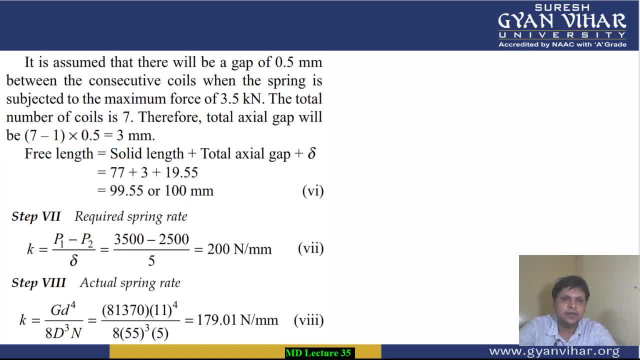 we have taken the value 100 mm. Then, coming into the next step, step number 7.. In this step we are going to calculate the spring rate. Now, in the spring rate, we all know, it is equal to load by deflection. But again here the load which we will take will be the difference of the 2 maximum and 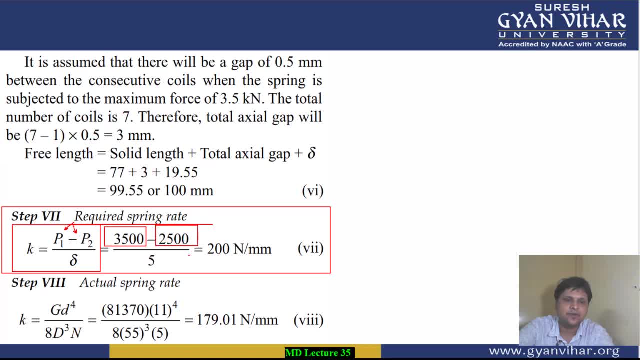 the minimum load, 3500 minus 2500, divided by the deflection value. Alright, So this we always keep in mind. here we will not take the maximum value of load. We will take the difference of the load P1 minus P2 by. 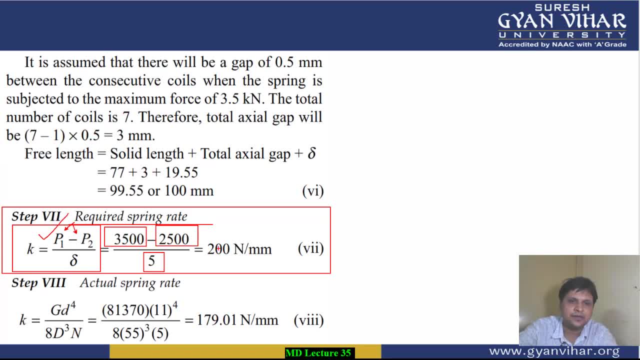 del. Alright. So this will give you the value of spring rate as equal to 200 newton per mm. It is not per mm, It is per mm square. Corrected, It is per mm square. Alright, Then the next step. 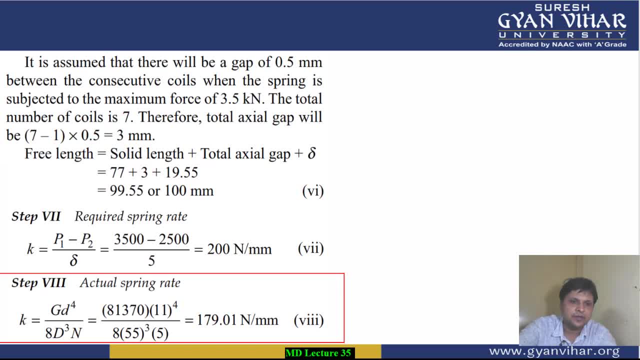 is actual spring rate. How we will calculate the actual spring rate? Actual spring rate can be calculated by the formula We all know. the formula for actual spring rate will be: k is equal to- We already know it is equal to. k is equal to P by del Alright And del equation: we already know it is. 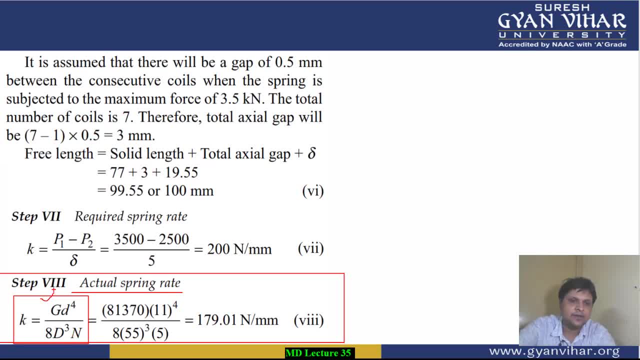 equal to. By this we can get the spring rate. formula k is equal to gd, to the power 4 upon 8 d cube n, Putting all those values, Because we already till now have calculated all the values. So including all these values, now we can get the. 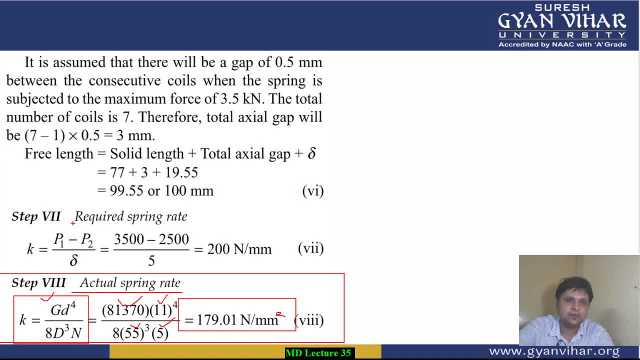 value of actual spring rate. This is the required spring rate which we need. But actually the value of the spring rate as given by the values which are given in the equation is this one. Alright, Don't get confused. This is the actual spring rate And this is this is the required spring rate which we have calculated. 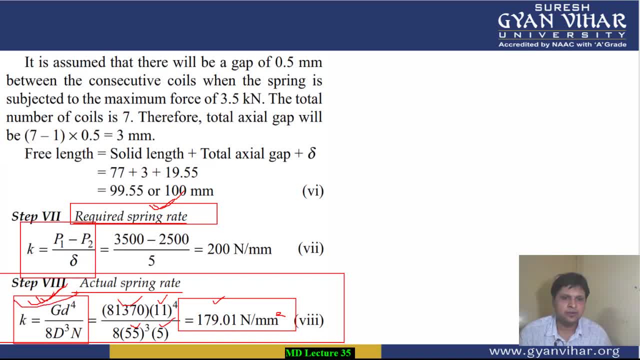 by this formula- And this is the actual spring rate- k is equal to gd, to the power 4 upon 8 d cube n. So you can see there is difference between these two values which we have calculated. So this was the numerical. So in this way we have solved the numerical. Now let's discuss some multiple. 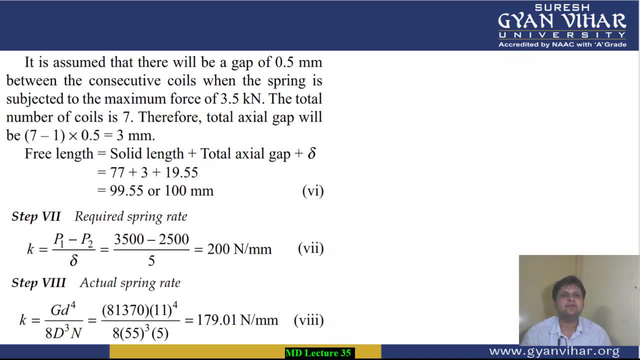 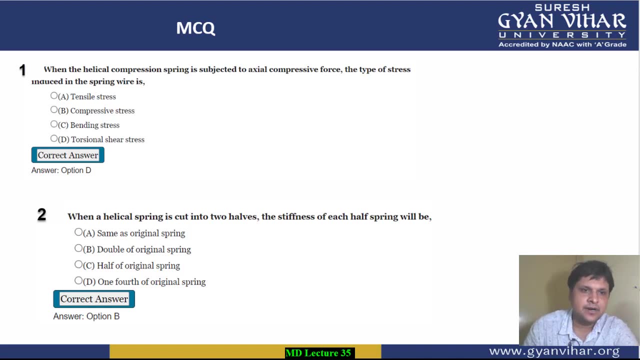 choice questions, students, in order to assess how much we have gained till now by discussion in this video lecture. So here are our multiple choice questions, Students. we will start with our multiple choice question number one, So let's read out what is our first question. When the helical compression spring is. The question is seeing us that When the helical compression spring is subjected to axial compressive force, the type of stress induced in the wire, so the type of stress that is induced in a wire when a helical compression spring is subjected to axial compressive force, is basically your what it. 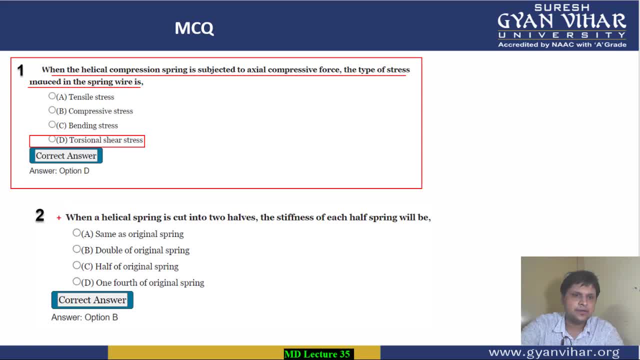 is the basically your torsional shear stresses. it is what it is. your torsional shear stresses very easy, numerical, very easy to mc multiple choice question. coming into the second multiple choice question, when a helical spring is cut into two halves, the stiffness of each of the half of 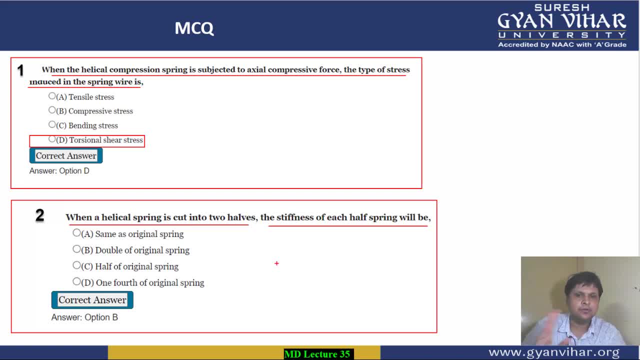 the spring will be. so if you will cut a helical spring into two halves, always keep in mind that the stiffness will not get half. it will be doubled because if the stiffness is basically equal to, if you for a case of a parallel spring, for a case of parallel case of spring, the stiffness is added. 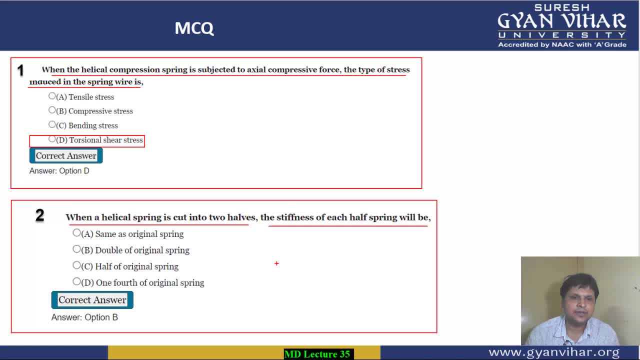 all right. so k is equal to k 1 plus k 2. so basically, what will be happen? the stiffness when you have cut a spring into two halves- it is stiffness- will remain same, and when you have- uh yeah, the half of this, the spring, stiffness of both of the half will be double. so option b is the correct option, that the stiffness 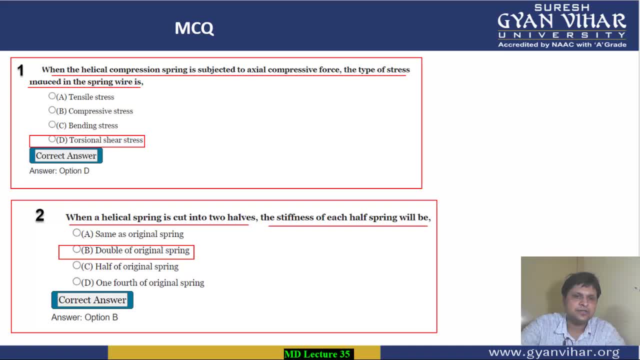 of each half spring will be double of the original spring. all right, so b is the correct option. all the other options, same as original spring, not correct. half of original spring not correct and one fourth of the original spring is not correct. b is the correct option. coming into the next multiple choice question, the type of spring, 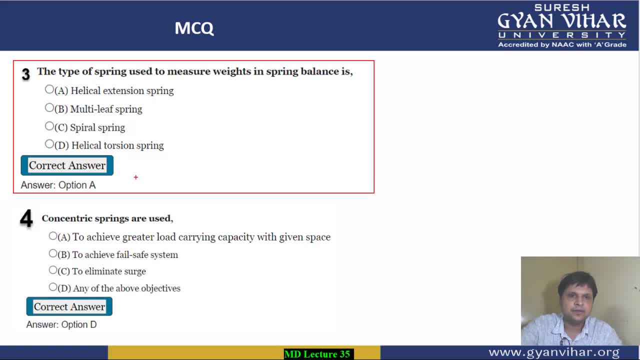 used to measure weight in spring balance is. so, in order to measure weight in spring balance, which type of spring we use? see, as i have already shown to you, if in spring balance you are weighing something, means you will attach something here, and this is the spring. so basically, the tensile load is acting on it. 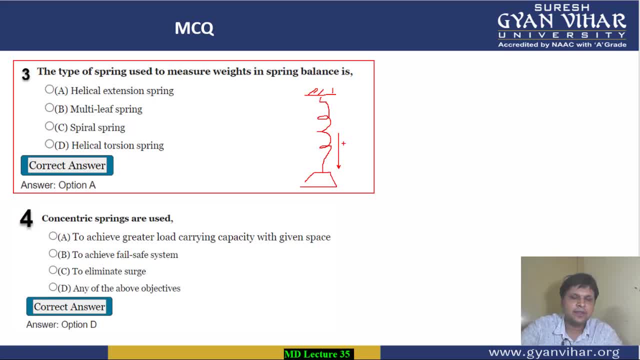 and the spring which we basically use is your extension spring. tension spring means you are applying the tension load, means the spring is your extension spring, all right, and basically the form of spring which we are using is the helical. so the option, first option, helical extension spring. this is very suited with the question. apart from this, the 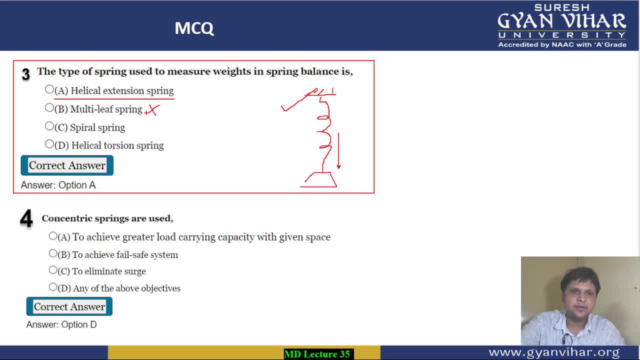 other springs, like multi-leave spring that is used for heavy compressions, then spiral spring. no, it is also not correct because you have a spiral springs are used in watches. then the third one is helical torsion spring. no, this is used in the doors, all right. so the helical extension spring. 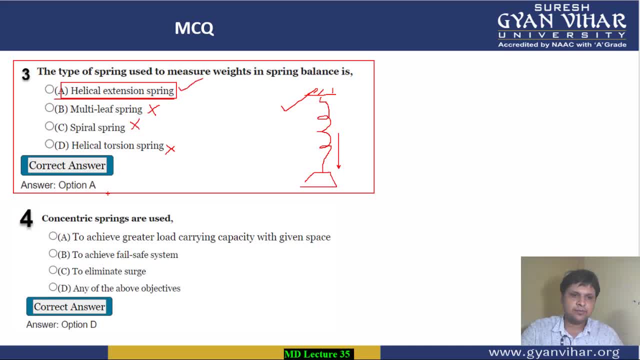 is the correct option. option a is the correct option of multiple choice. position number three. all right, coming into multiple choice, question number four, springs are used in now. concentric springs means which are having the same axis. this is the spring. there is one more spring like this. let me change the color of the spring so that you can understand. 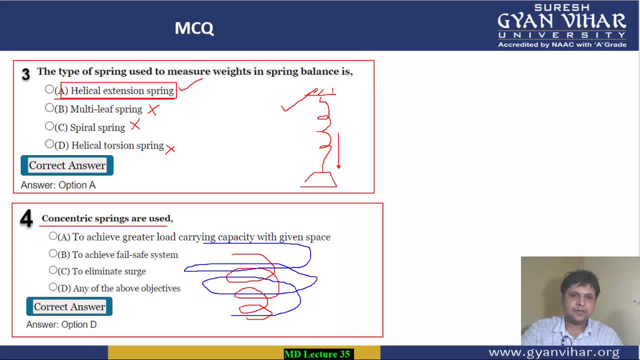 better. this is the other spring. now both are having the same axis. both are having the same axis, so such type of springs are known as concentric springs. i will tell this particular type of spring in the next video lecture in detail, and in concentric springs are basically used. 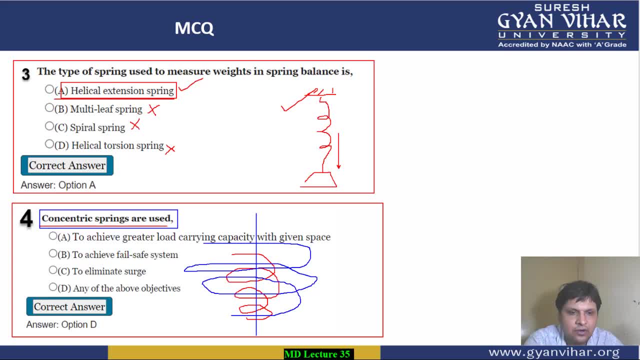 in order to increase the load carrying capacity of the spring. if we want to increase the load carrying capacity of the spring, then in that case we use the concentric spring. so here in the options, let's read out what are the options. first is to achieve greater load carrying capacity. 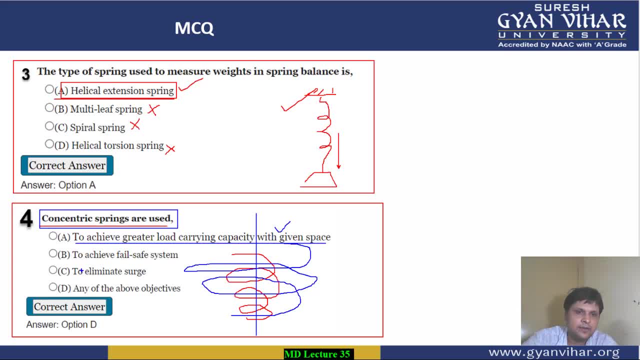 with given space. so this is the correct one among parts. let's read other also: to achieve fail safe system. this is also correct. third one: to eliminate the surge in spring. this is also correct. so if all the three options are correct, then d, which is saying that any of the above objective is the correct means. d is the 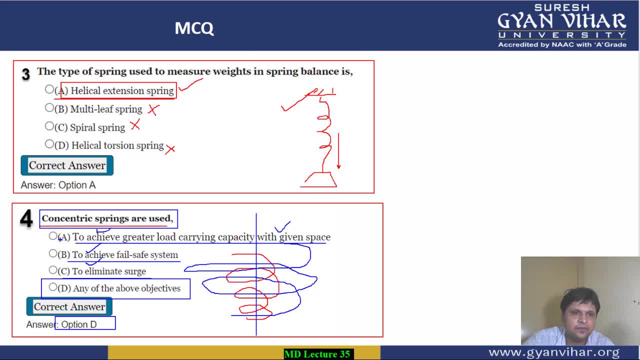 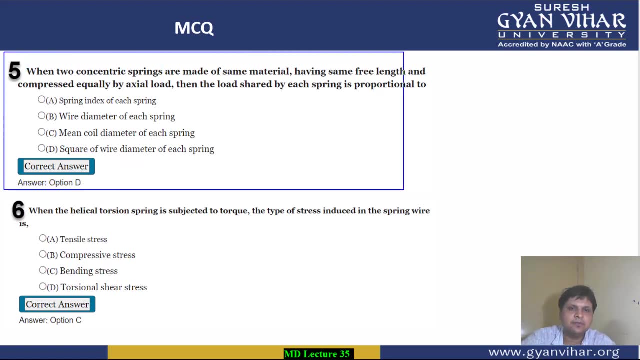 correct option. all these three are the benefits of concentric spring: greater load carrying capacity, fail safe operation and the elimination of surge. coming into the next multiple choice question, number five, when two concentric springs are made of same material, having same free length and compressed equally by axial load. 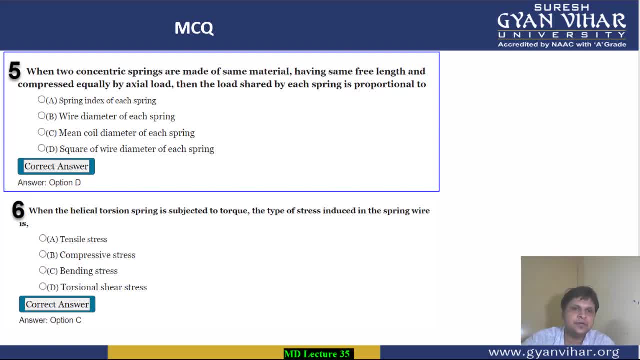 then the load is shared by each spring is proportional to. so if the material is same, free length is same and compressed length is also same of two concentric springs, all right then the load shared by each each spring. i will tell you in detail in this coming lecture. also the load. 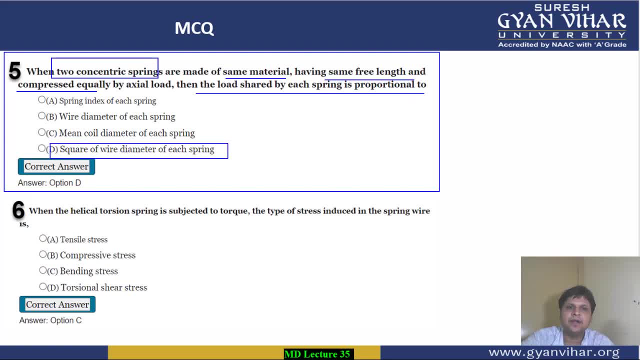 shared by each spring is squared of wire diameter of each spring. apart from that, is load is proportional to spring index. not the correct answer. wire diameter proportional. no mean diameter proportional. this is also known. so option d is the correct option. coming into multiple choice, question number six, when the helical torsion spring is subjected to torque, 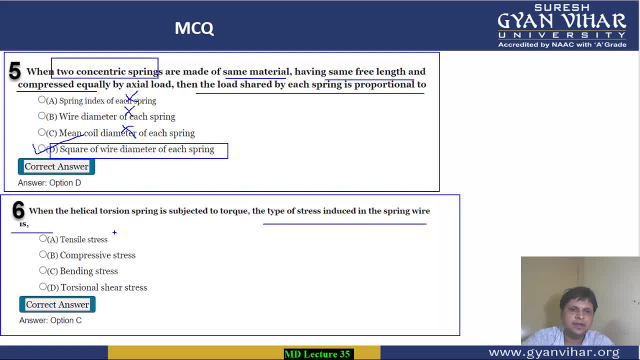 the type of stress induced in the spring wire is so helical torsion spring is subjected to torque. the type of stress that is induced in the spring wire is basically your. this is a question in which you can get confused: the type of load that is acting in the spring. 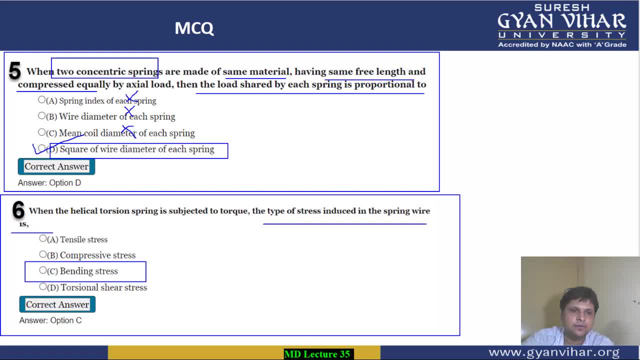 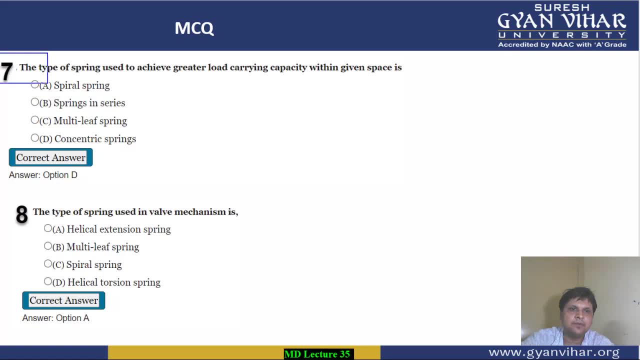 wire is your bending stress. all right, bending stress is the type of load, so option c is the correct option. coming into multiple choice, question number seven: the type of spring used in interest, not is the type of spring used in ironing to achieve greater load carrying capacity within given space. so this i have already told you. for higher load carrying ability you use, 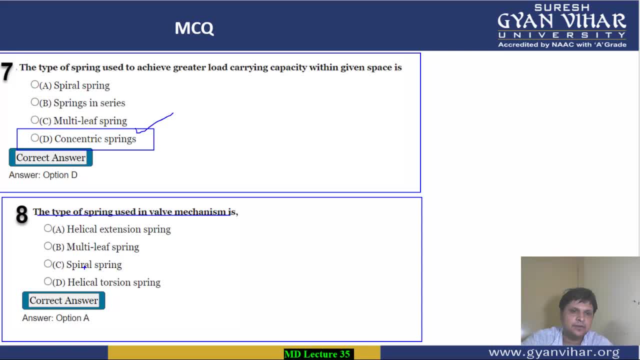 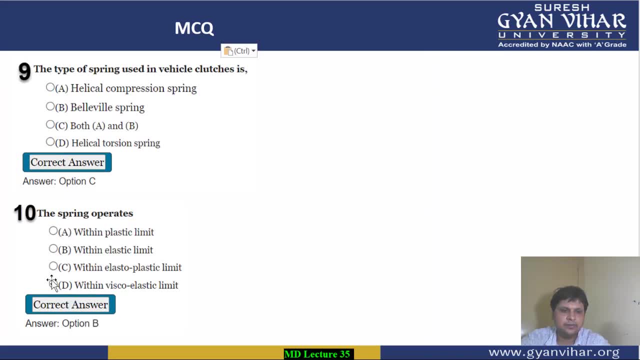 the concentric spring. d is the answer. eighth number question: the type of spring used in wall mechanism is so in wall mechanism we know that helical extension spring is used. option a is a correct option. coming into multiple choice question number nine: clutches of the vehicle. the spring that is used is also helical compression spring and 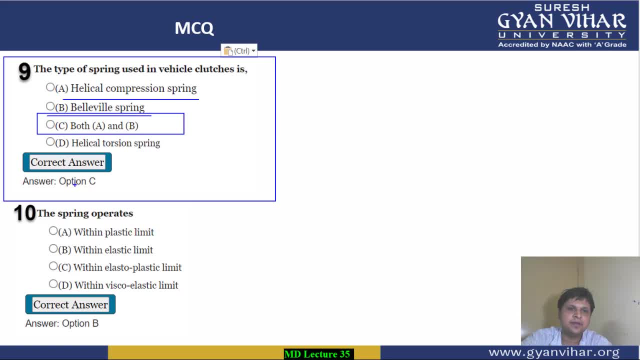 believable spring, so both a and b is the correct option. coming into multiple choice question number 10, the spring operates. we all know that spring operates operates within elastic limit, so b is the correct option. so all the multiple choice question we have discussed is the content which. 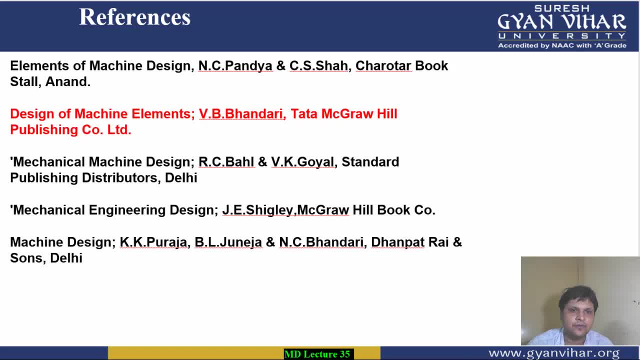 i have prepared to make you learn about this topic was from these references. you can also use these references for your self-study students. for today, this is enough. thank you students. thank you and have a nice day.